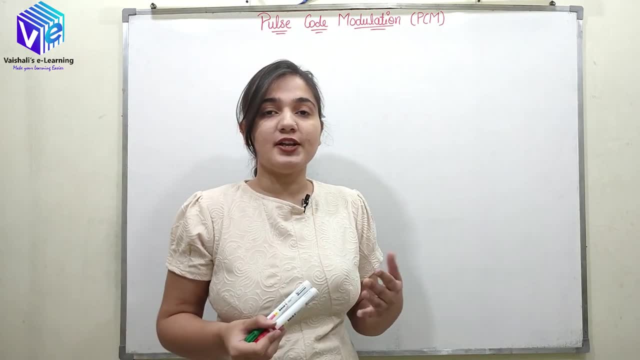 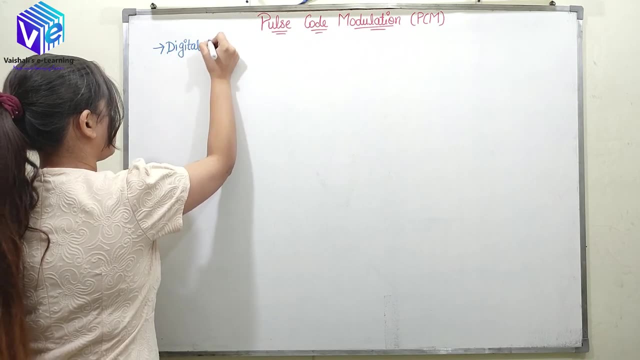 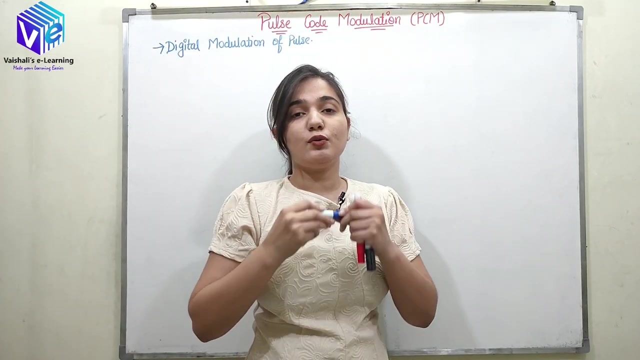 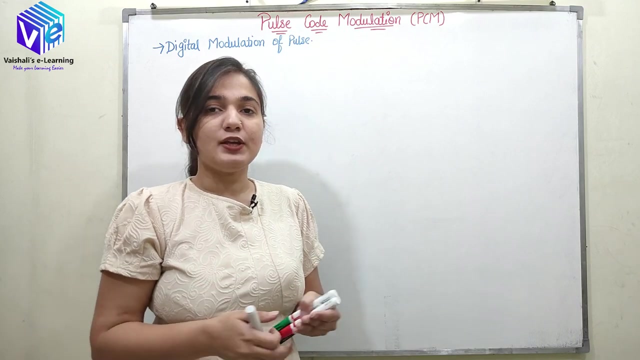 said, it is the digital modulation of the pulse. So now, if I ask you, what were we doing in the sampling? We were changing the analog time to discrete time. So now here, a main part of this pulse code modulation technique is that we are going to talk about the pulse. 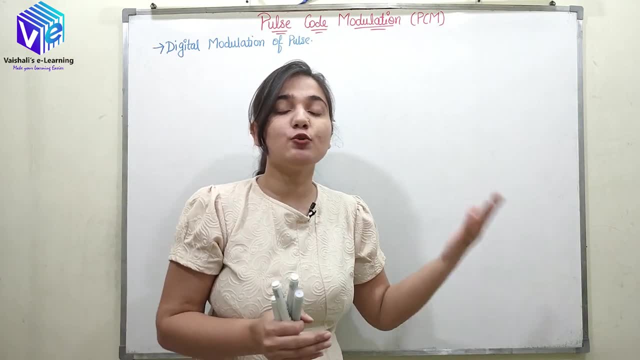 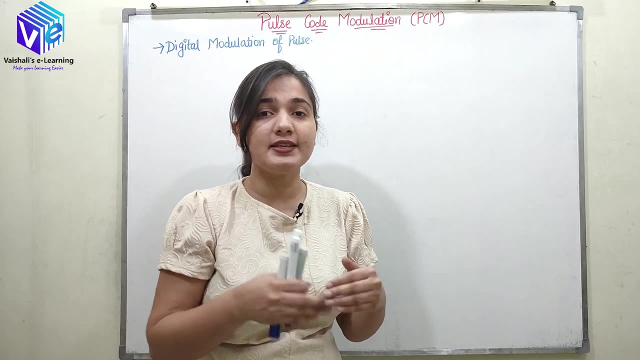 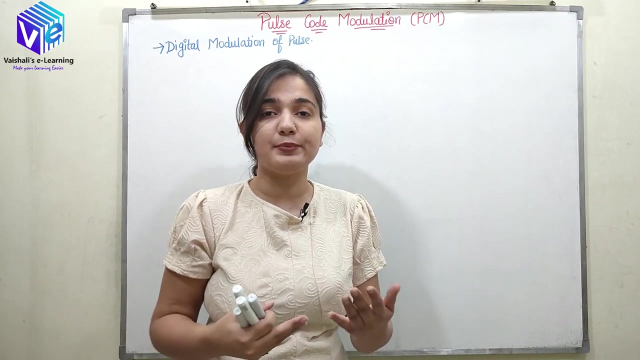 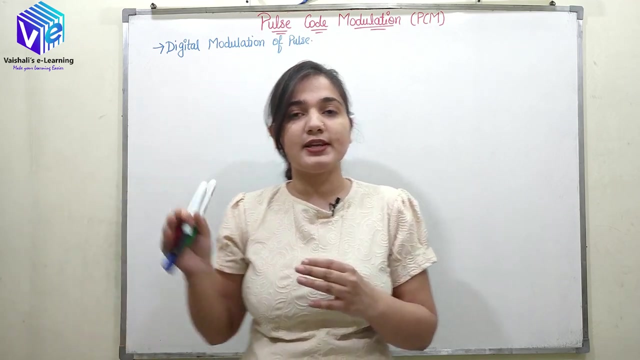 code. modulation technique would be sampler. After that we have a quantizer. So, like the way we were changing the analog time axis into discrete time axis, in the similar way I can change the analog amplitude axis into discrete amplitude axis and the process is called quantization. After that we have discrete levels. we can encode these levels with different. 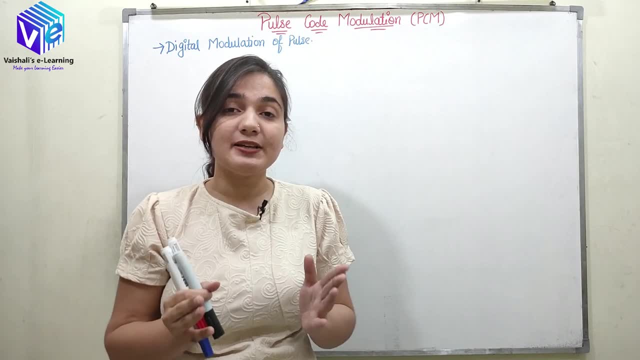 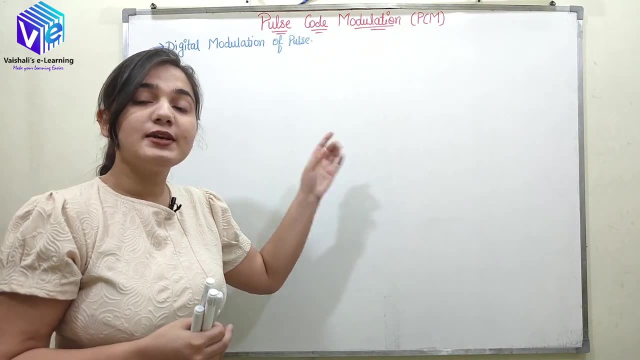 bits. So now these bits are quantized. So now we are going to talk about the pulse code modulation technique. So these are called digital bits, and these bits are always in the form of zeros and ones. So now, here in this process, we are sending the zeros and ones, so it is a digital. 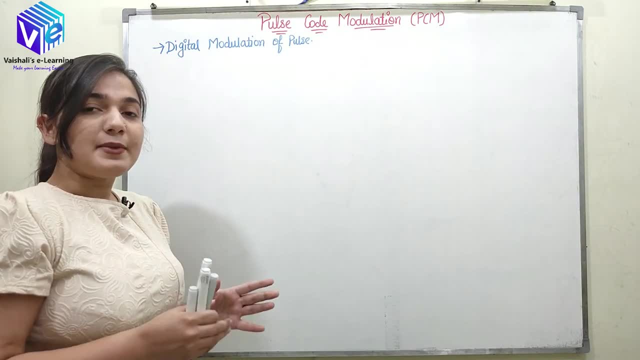 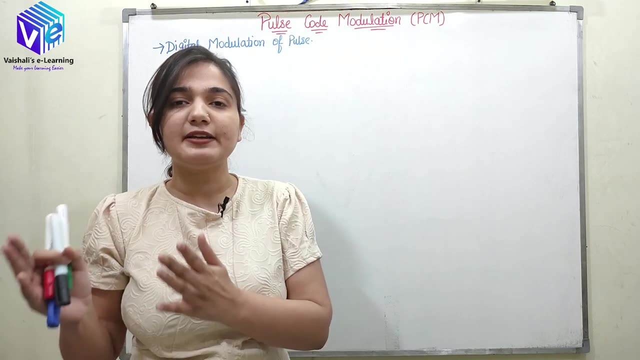 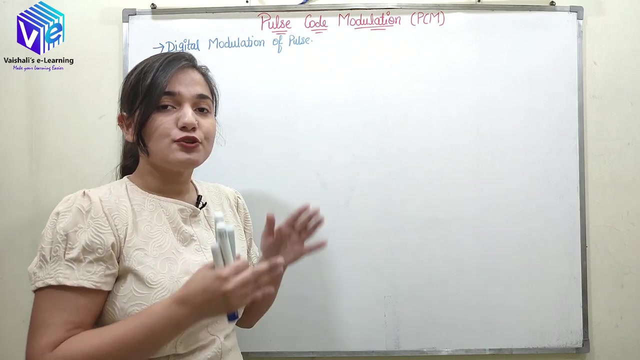 transmission. So let's see the block diagram- and we will be discussing all of the blocks in the block diagram of the pulse code, modulation and demodulation techniques. We will be talking about the channel as well. So we will be having three different blocks. So the first one is: 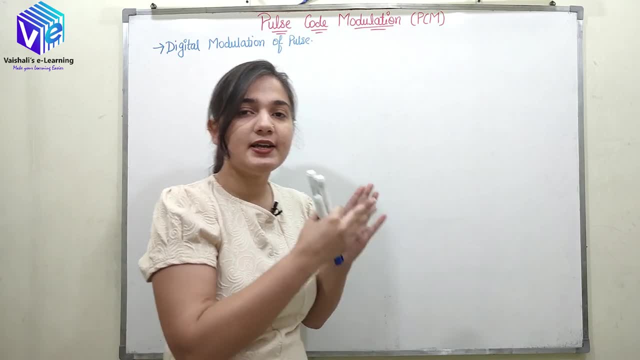 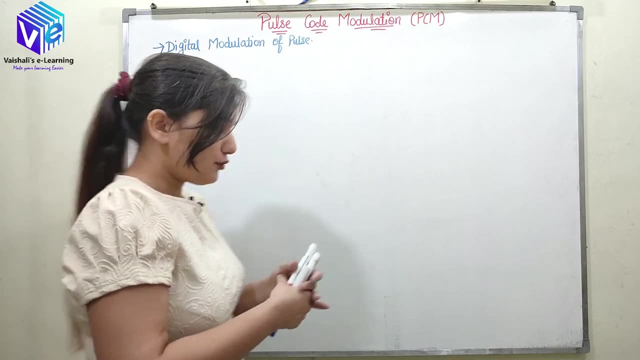 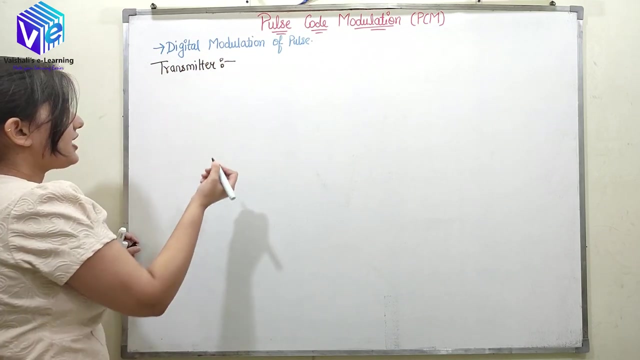 type of block diagram would be the transmitter. Second, we will be seeing what happens in the channel and at the last we will be seeing what happens at the receiver. So now, if I talk about the transmitter, So in the transmitter, the first thing I will be having is the source. 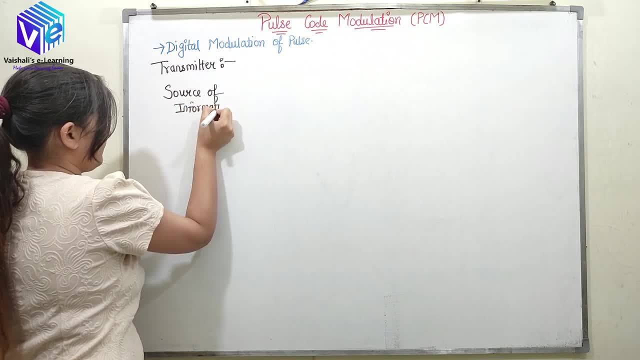 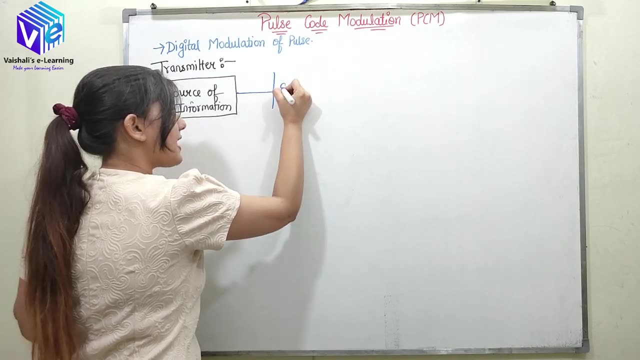 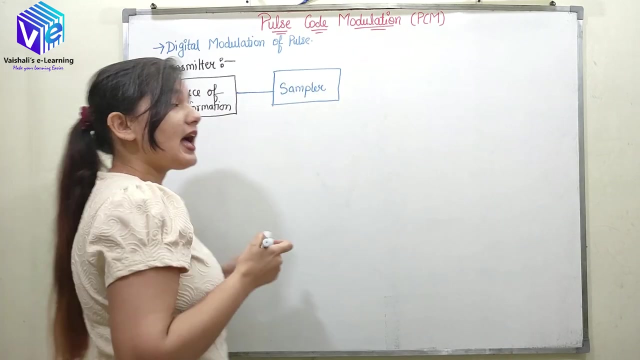 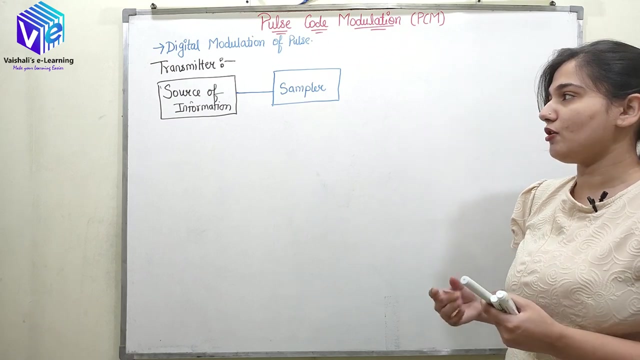 of information. It is connected to the sampler. The source of information is always giving the information in the analog form, So remember this. the most of the signals in the nature are generated in the form of analog signal. So here I will be having an analog signal. After that it is passed to the 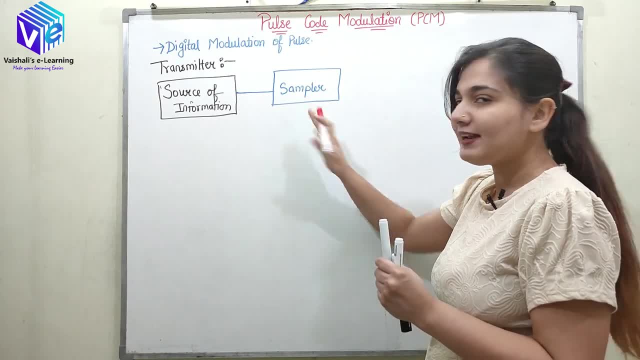 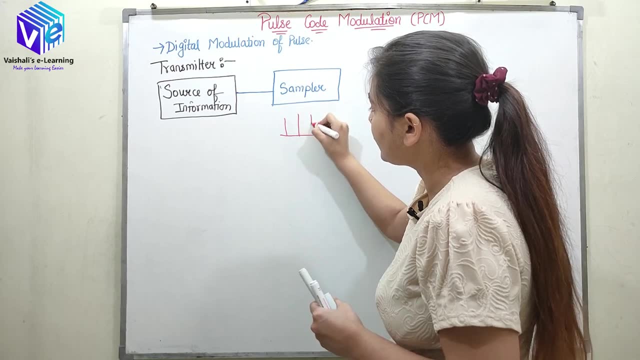 sampler. I hope you are very pro in the sampling and you know what happens in the sampling. So here we are converting the analog signal to the sampler. So here we are converting the analog signal to the time axis into discrete time axis. So I hope you remember this. If not, you can go and watch the. 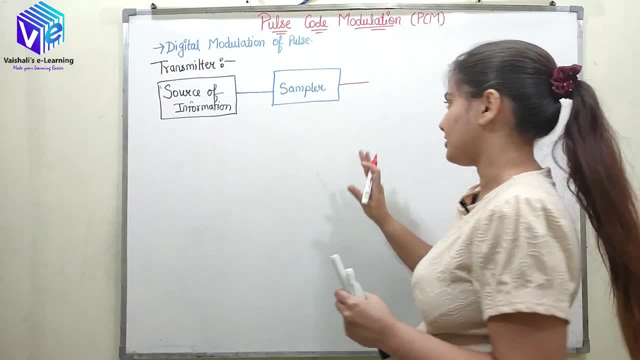 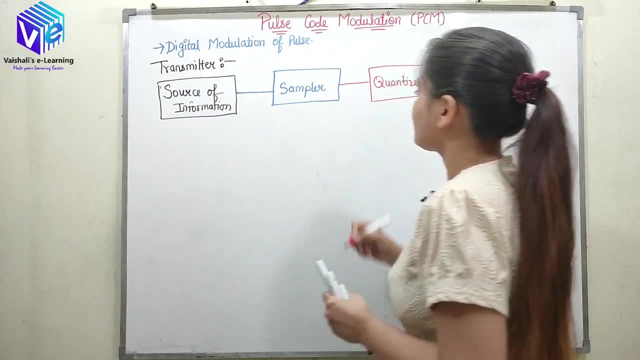 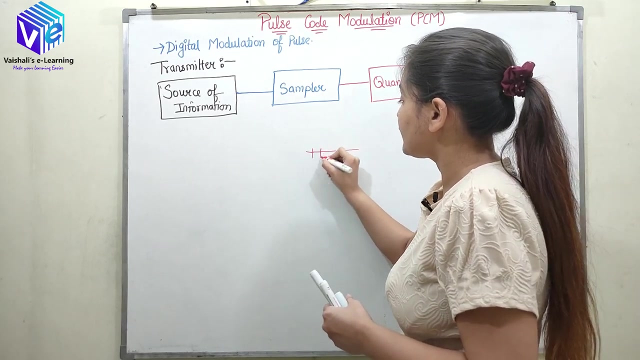 previous video on sampling theorem and its reconstruction as well. So now here, after that, we have quantizer. What is quantizer Like the way sampler is converting the time axis into discrete levels. Here it is converting the amplitude axis to the time axis. So here we are converting the 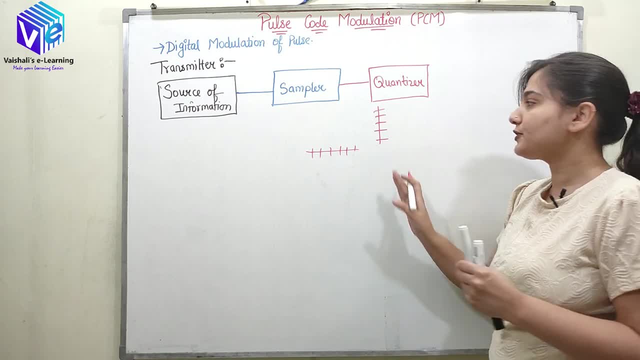 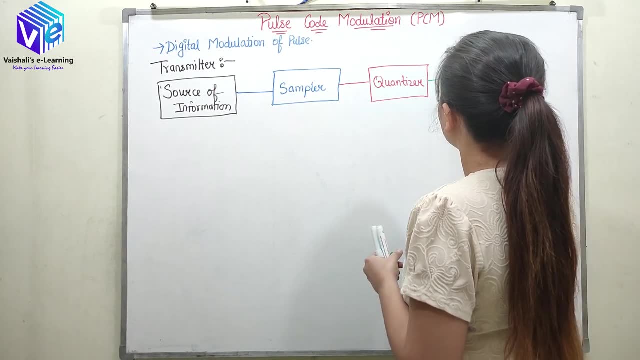 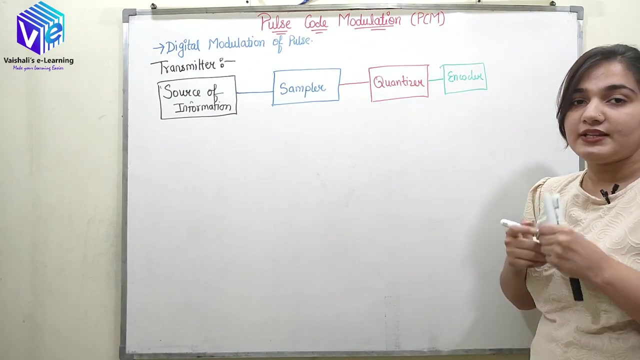 time axis into discrete levels. We will be talking about it in detail. So now, after that, we will be having an encoder. Encoder is converting the discrete levels into digital codes. So these discrete levels are converted into codes in the form of zeros, and once only. So here I will be. 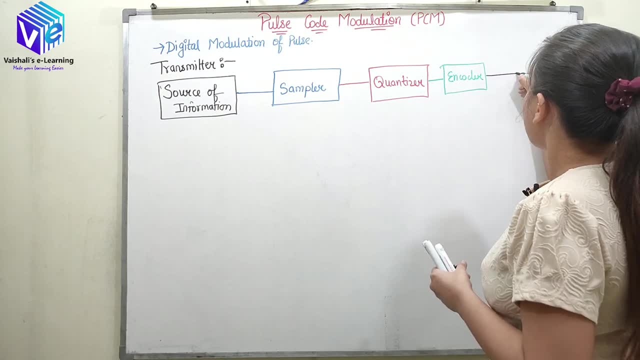 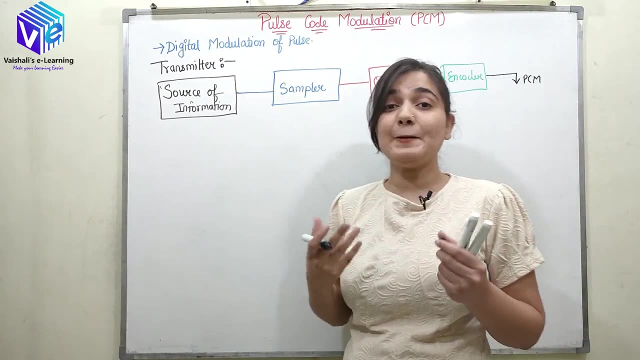 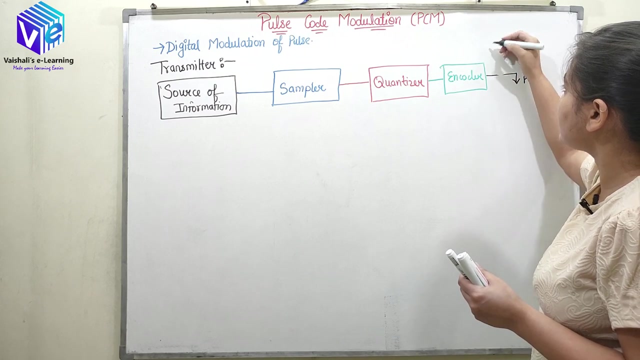 getting a digital signal. So this is the pulse code: Modulated signal. So how it is? I am saying it to be a pulse signal. So now here the zeros and ones which are formed. So let's suppose we have a long series of data which is 0, 1 0, 1 0, 0, 0, 1, 1, 1.. 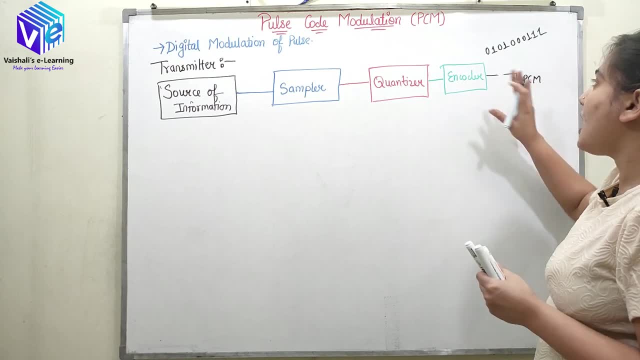 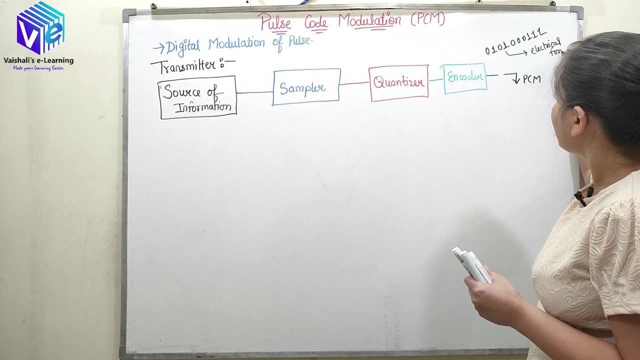 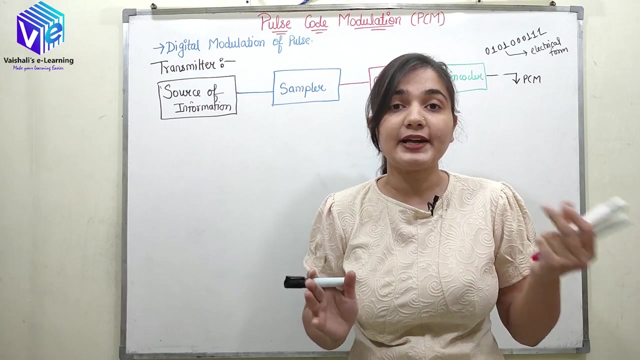 So this kind of data will come after the encoder. Now this data is transmitted after converting into the electrical form. So now I hope you remember I have already talked about the electrical form, The line encoding, The conversion of digital data into electrical signal. So here the zero is. 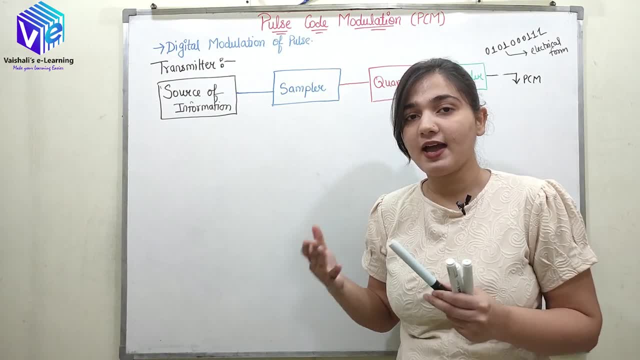 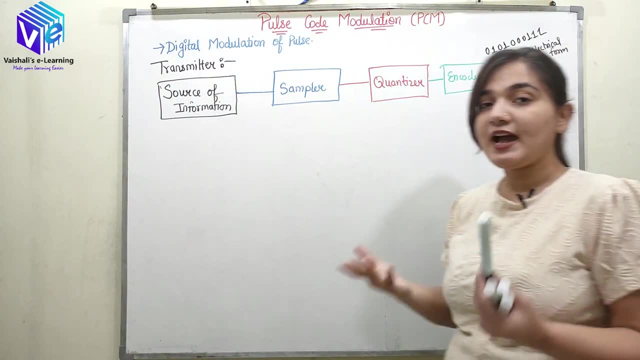 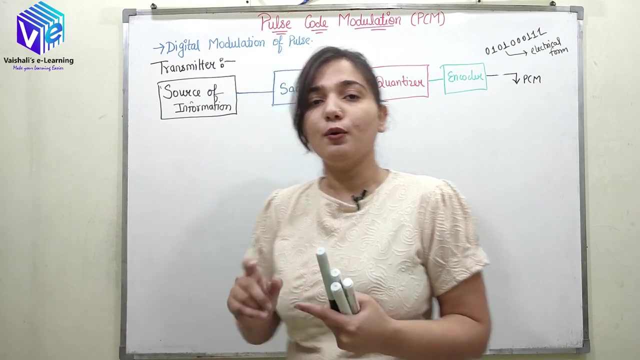 represented by some digital voltage and one is represented by another level of voltage. It is also in the form of pulse. So now, what kind of pulse is that? The amplitude is changing, No, Width is changing, No Position is changing, No, Only it is changing according to the data. 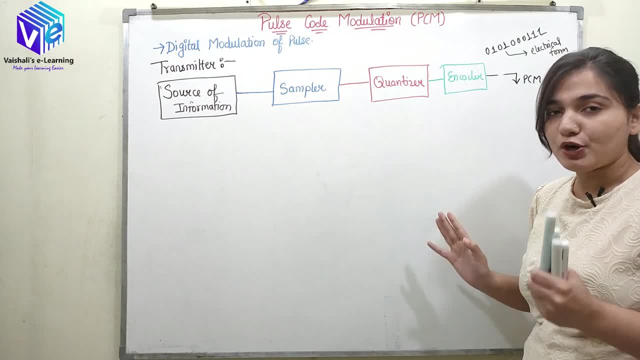 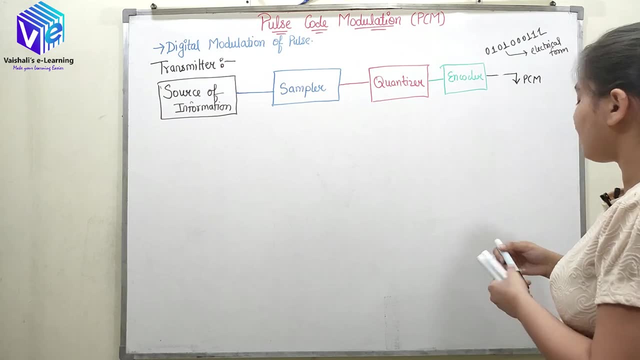 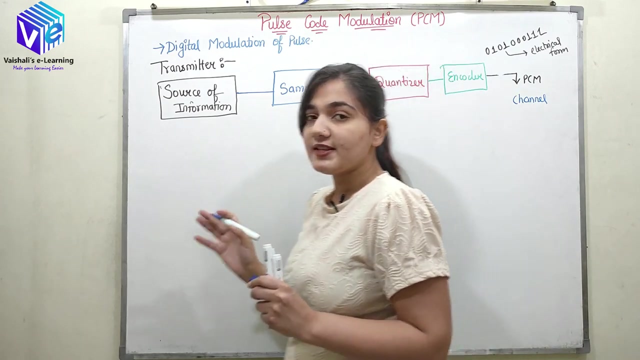 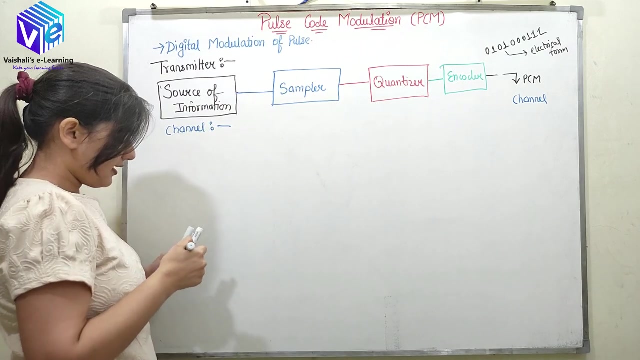 So now this is digitally Pulse code modulation technique. So I hope now you are very clear about the generation of pulse code modulation. So after that it is going to the channel. So now with the second block diagram would be about that channel, as I already told you. So the next thing I will be talking about is about the 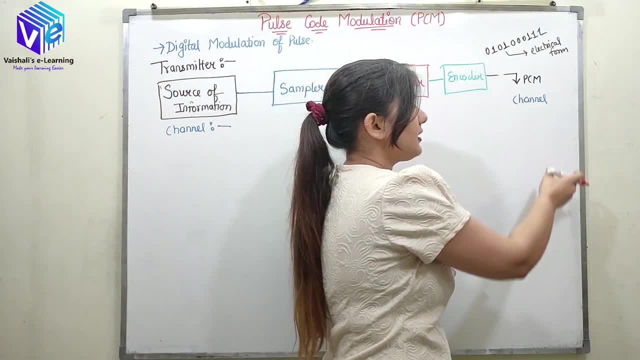 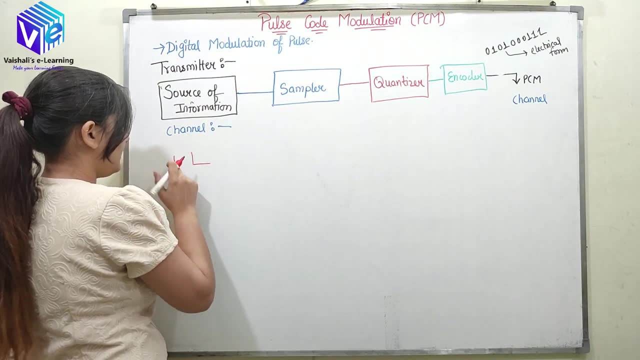 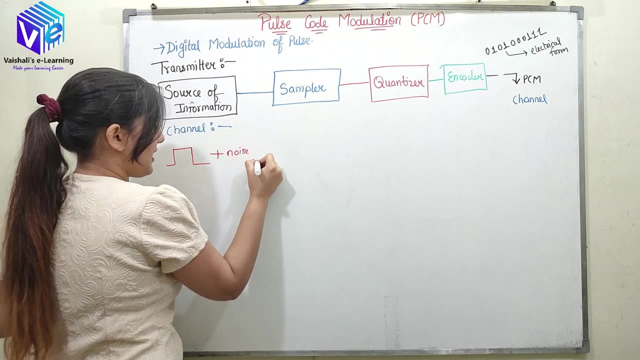 channel, So here in the channel, when the signal will come. So in the channel there are noises, So the signal was in the form of a digital signal, So it's in the form of a pulse. So this pulse is added with the noise and I will be having this kind of signal. So now this: 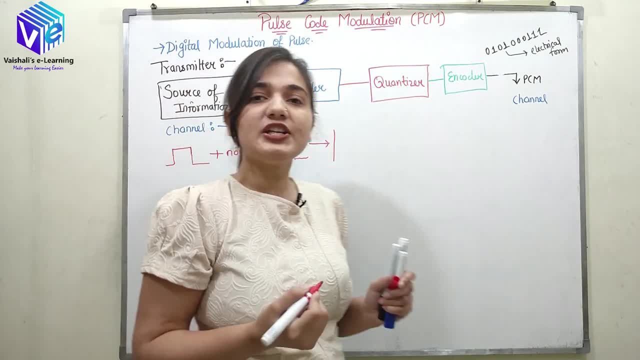 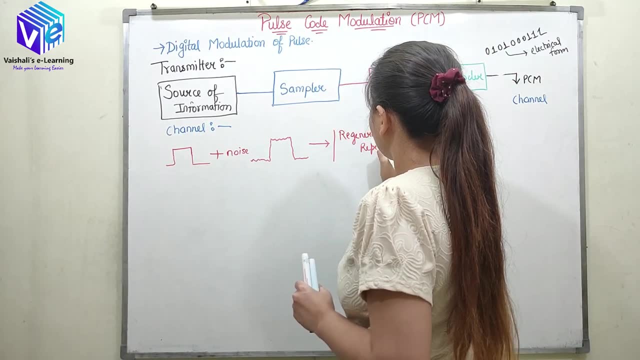 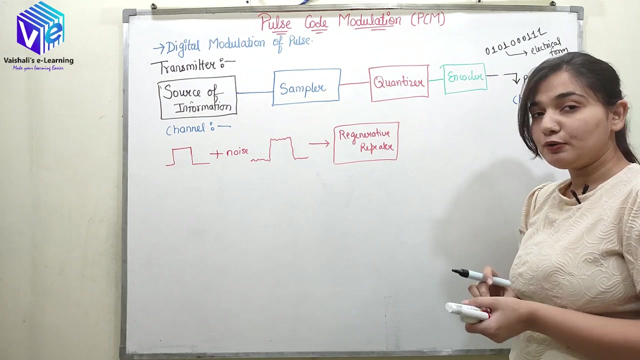 signal is fed to a series of regenerative repeaters. So let's understand this. So I hope it is clear That we don't have single regenerative repeater. We can have, Don't confuse with it. We can have multiple regenerative repeaters based upon the need. 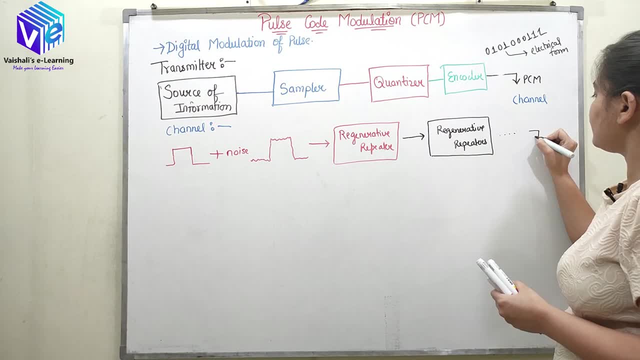 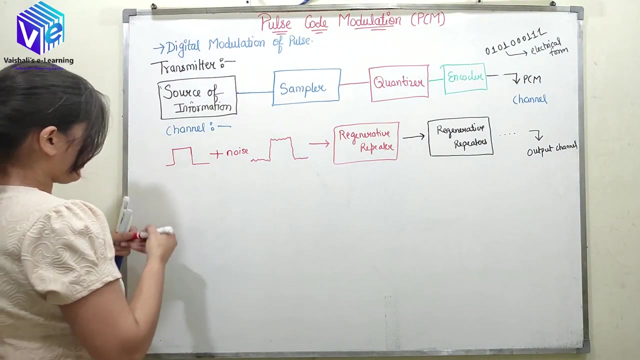 Now, if I have n numbers of regenerative repeaters. after that it is fed to the output of the channel or the input of the receiver. The output of the channel is the input of the receiver, obviously, So here we'll be talking about the receiver block diagram. 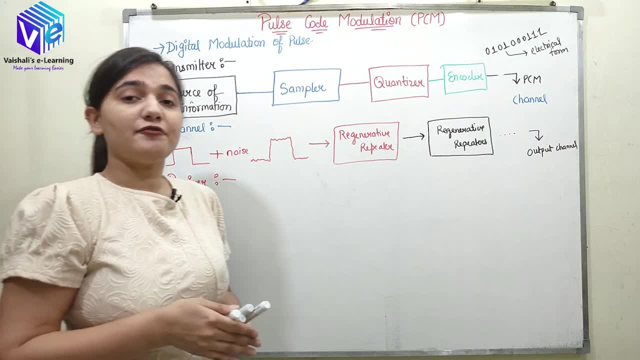 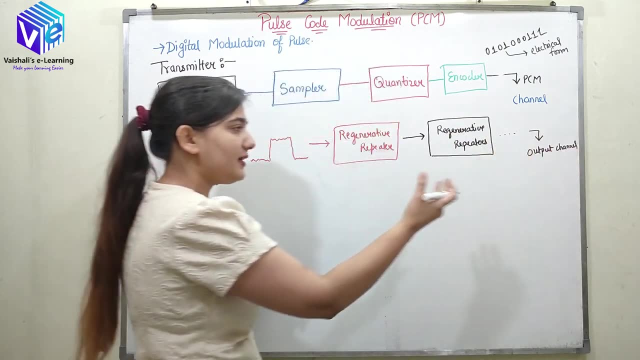 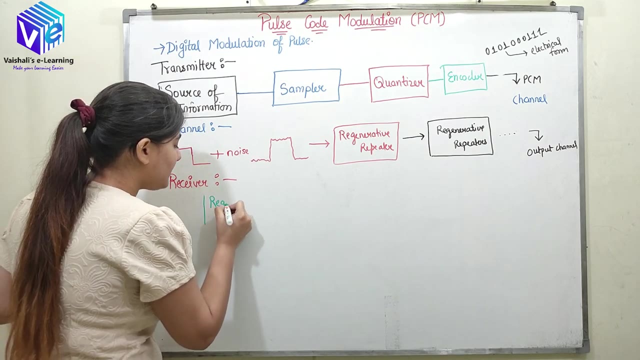 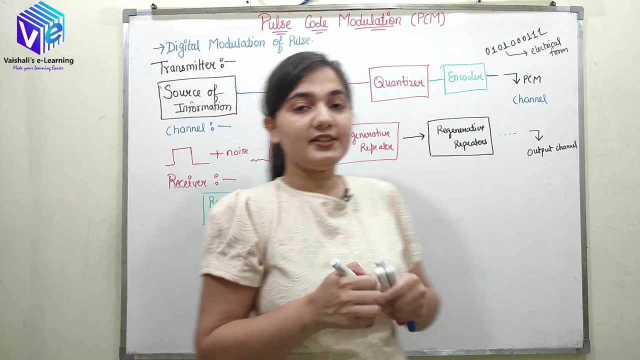 So now what happens? First thing in the receiver. So after we have repeaters, we have some space to treble. the signal石 get added. So first thing I'll be having is a regeneration circuit. So after that we are just converting my signal back. 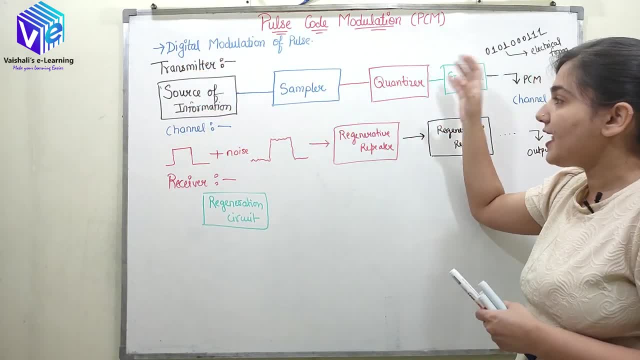 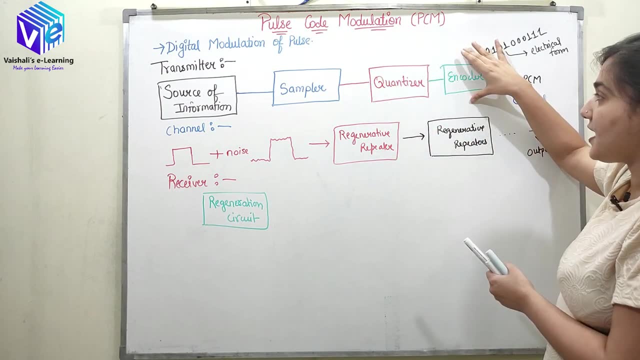 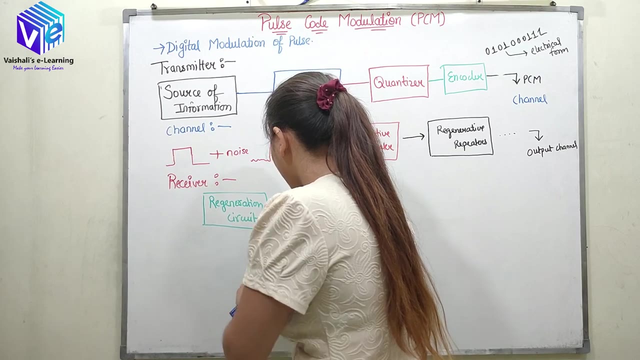 to this form in which the source sent. so I'll be doing all of the reverse of the things which are happening in the transmitter. So first I'll be using the encoding, So I'll be doing the reverse of encoding which is decoding. So here I have a 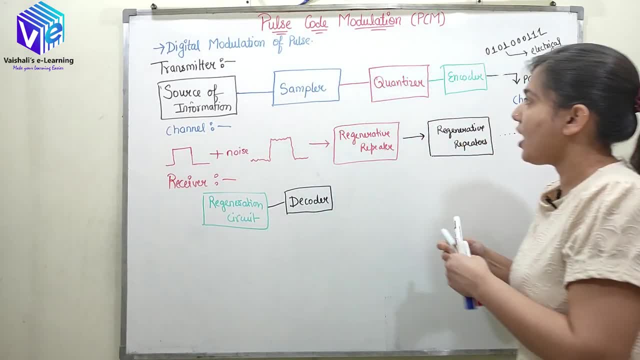 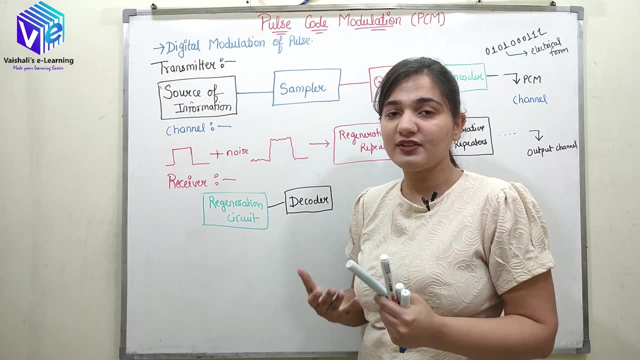 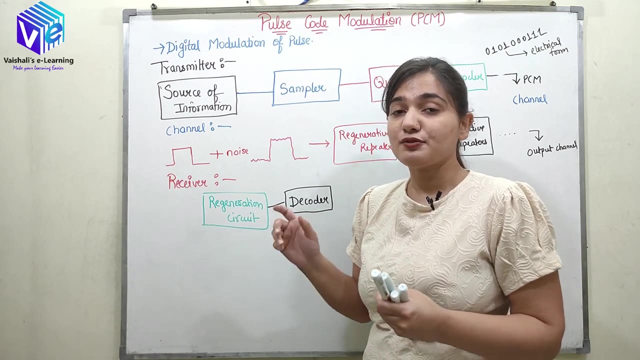 decoder. Okay, now, after that we have a quantizer, but we don't have any reverse of quantizer. So it's a negative thing for us And because of that there is a humming sound when you try to receive a random signal. So because the 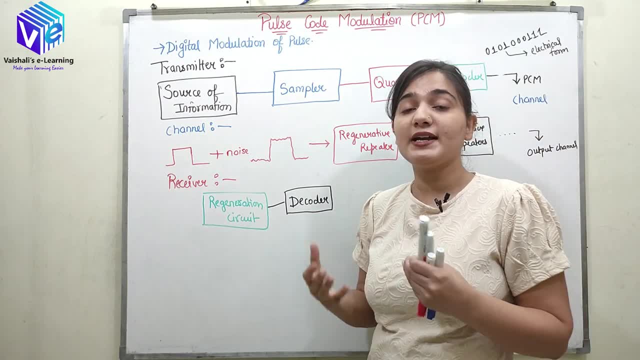 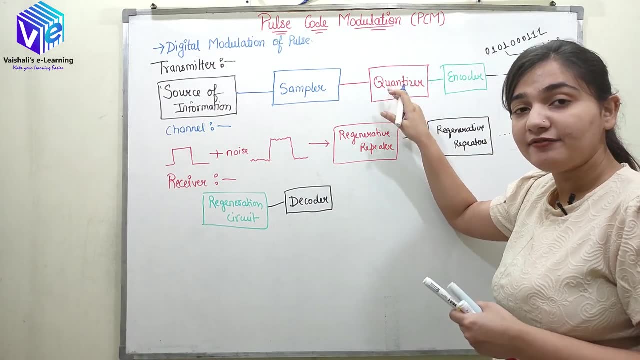 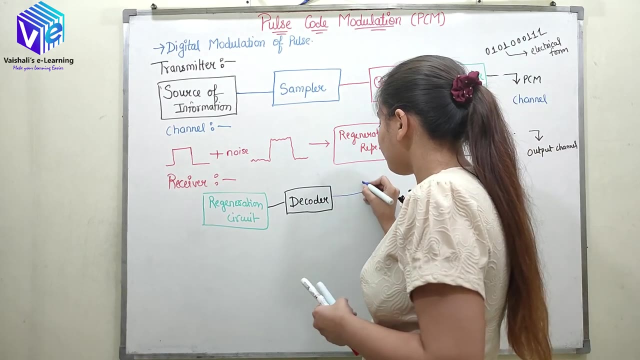 quantizer is producing an error, which is called the quantization noise or the quantization error. So now we cannot have the reverse of the quantizer. So now, moving to the next block, here we have sampler. So instead of sampler we have reconstruction filter. 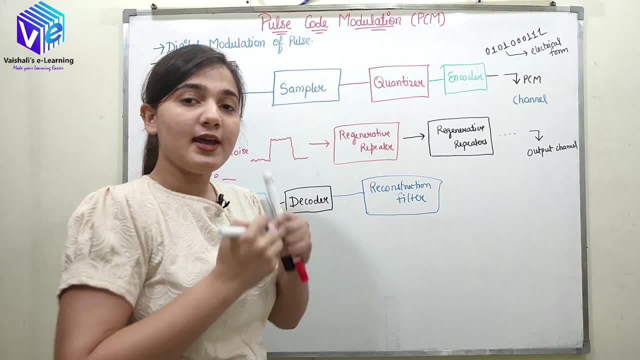 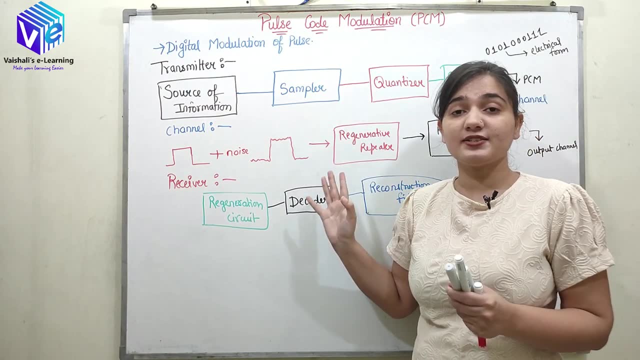 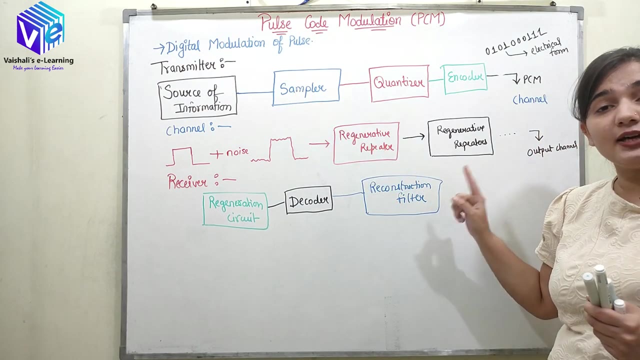 What is a reconstruction filter? I hope you remember it is a low pass filter. I hope you remember the reconstruction after the sampling. we can reconstruct the sampled out output with the help of a low pass filter. So here, to counter this, we are having the reconstruction filter. So now, 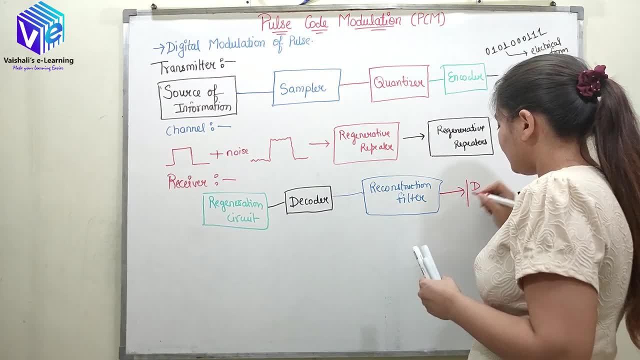 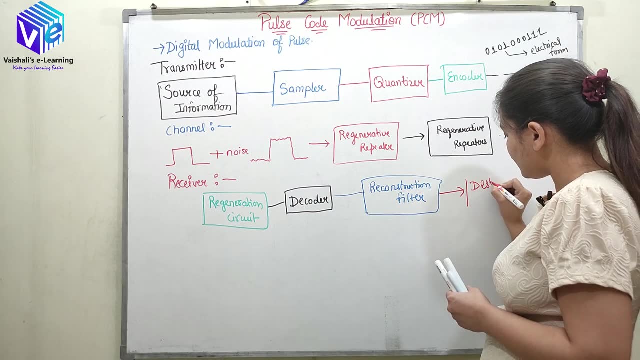 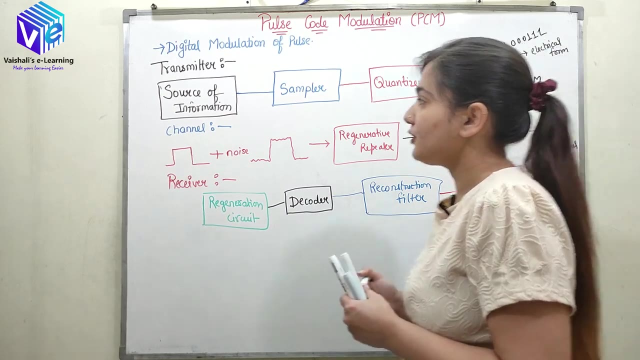 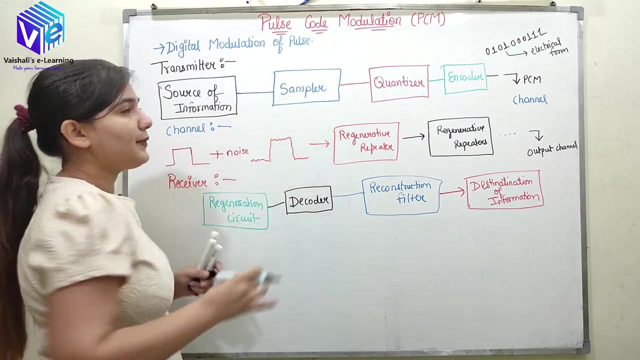 after that we'll be getting the signal in the form of the same form which the source sent. So here we'll be having destination of information. So now let's discuss in detail what all happens. So now, here before sampler, I have a pre processing block which is: 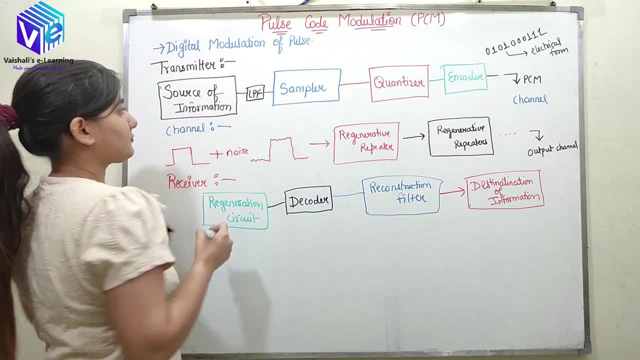 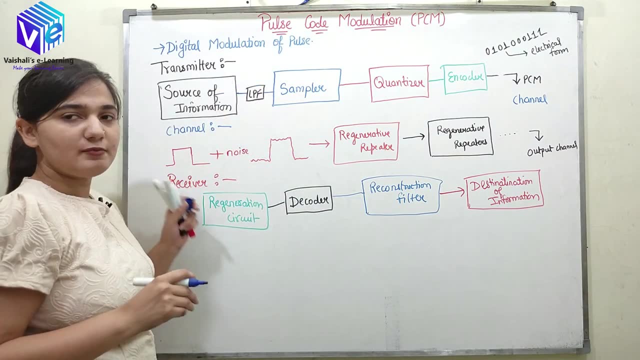 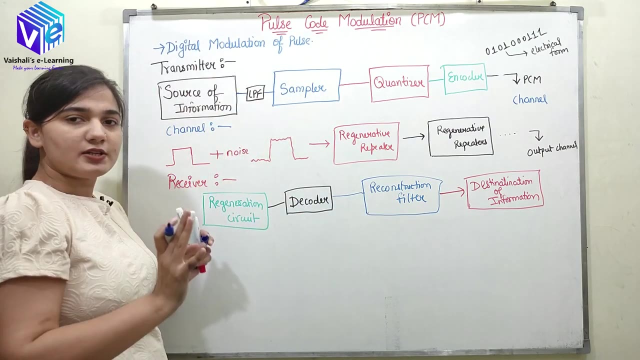 called the low pass filter. So now let's understand all of the blocks in detail. So first I have the source of information. I hope you know you are also a source of information when you are talking to some other person. So now the source of information is clear. So now, 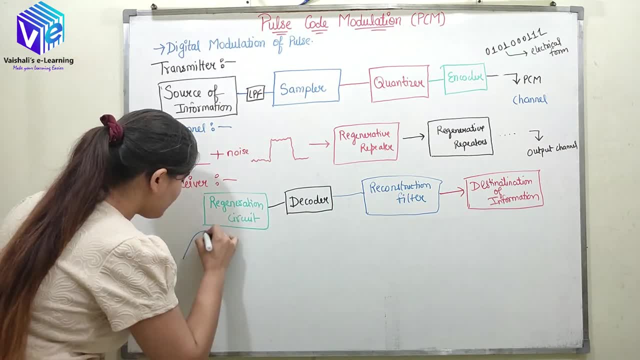 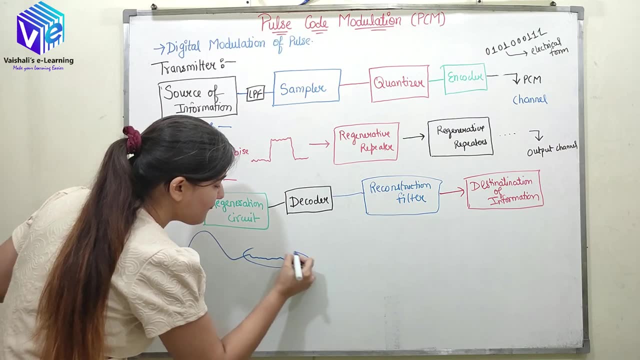 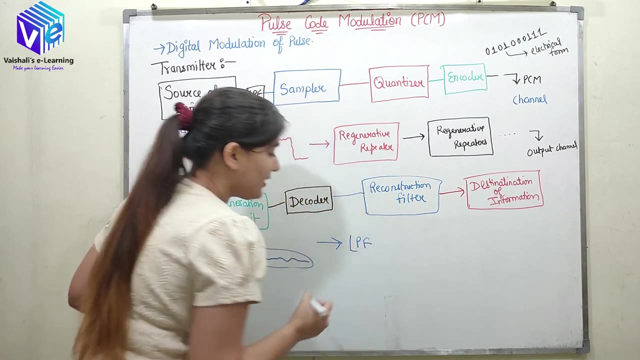 after that we have a low pass filter. So now the source of information is producing some signal in this form. So now here we have some high frequency signals as well, So this signal is passed to the low pass filter for band limiting. I have already talked. 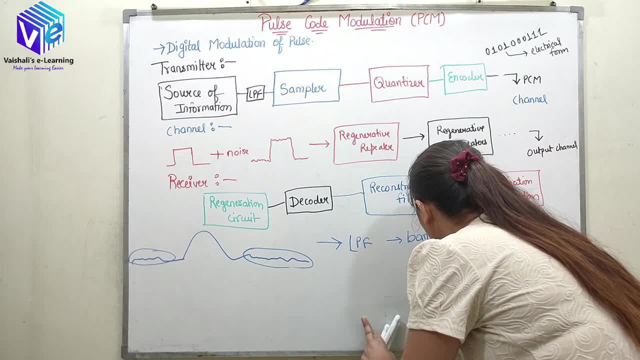 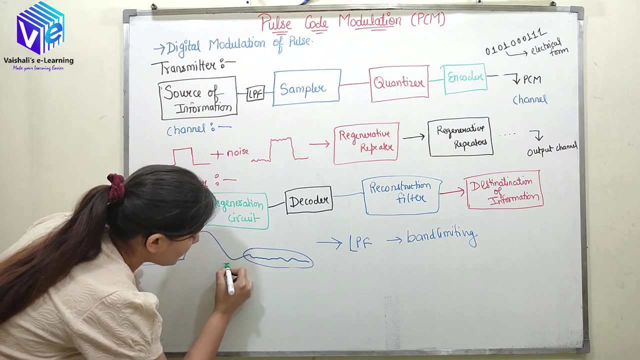 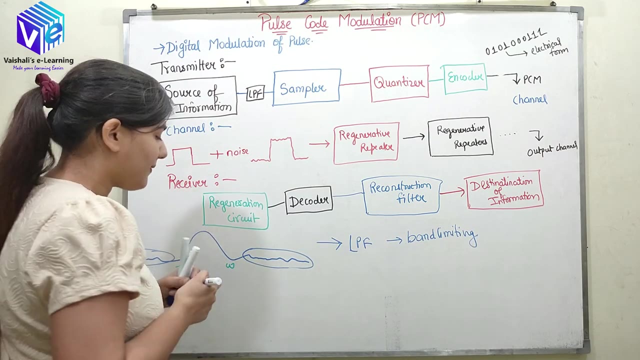 about the concept of band, limiting why it is required. So now here. the most of the major frequencies are present in the range minus W to W, or I can say minus FM to FM. These frequencies are ranging up to infinity and these are carrying very less. 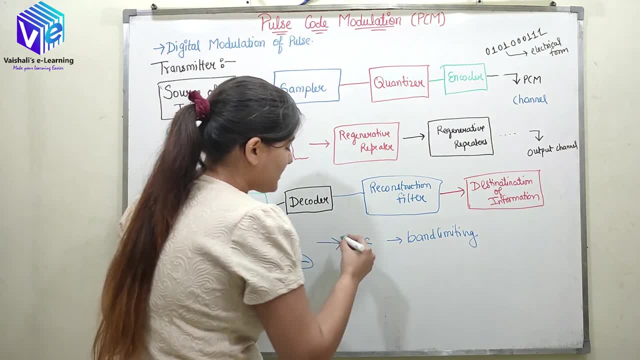 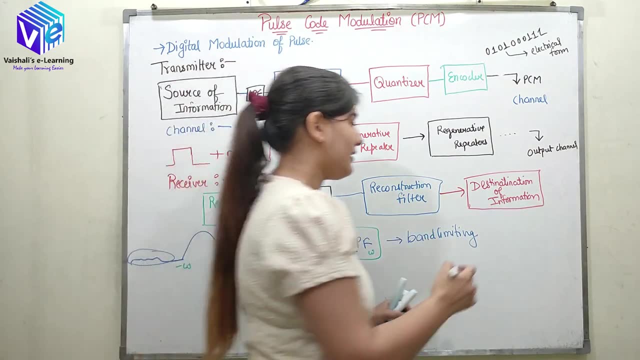 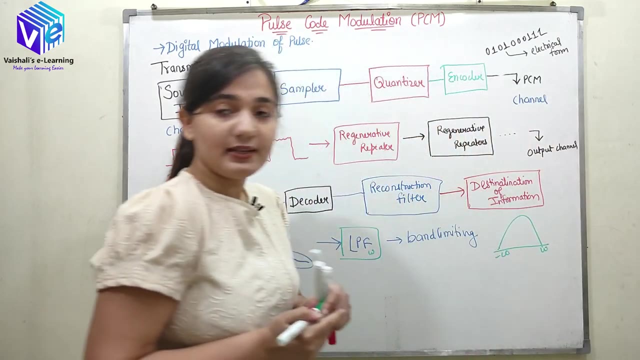 information. So what I'll do? I'll be having the low pass filter with the bandwidth W. So now here: if this signal is fed to the low pass filter, here at the output I'll be having the band limited signal. So why this band limited signal is required? 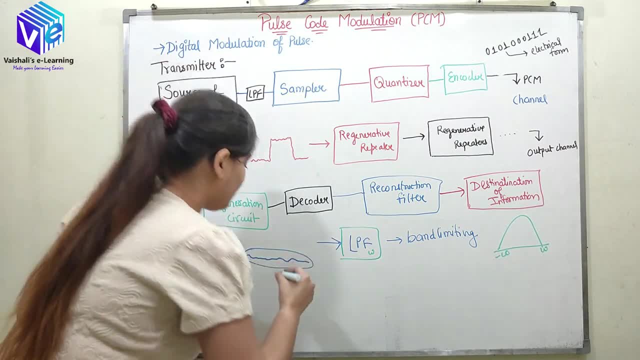 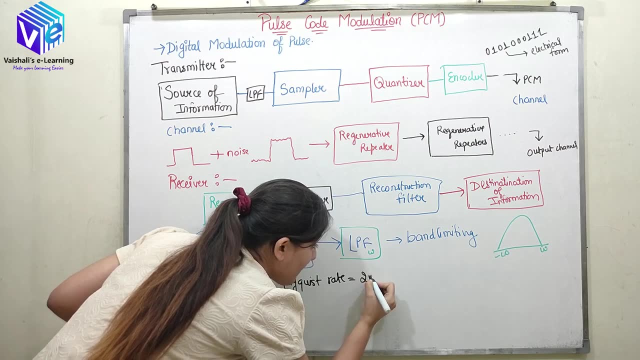 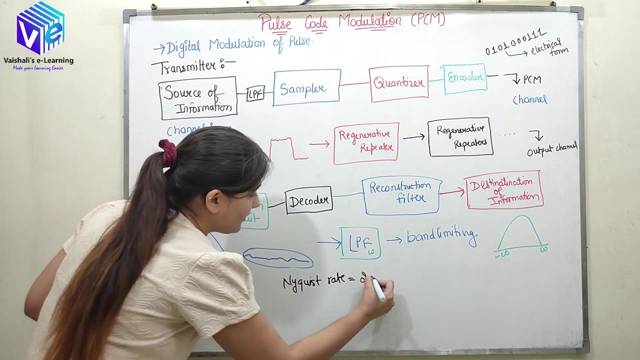 Because in sampling I hope you remember the Nyquist rate. Nyquist rate was twice into the maximum frequency. What is the maximum frequency here? So if I talk about this signal, so here I'll be having, so it is maximum frequency. So here, twice into infinity. So 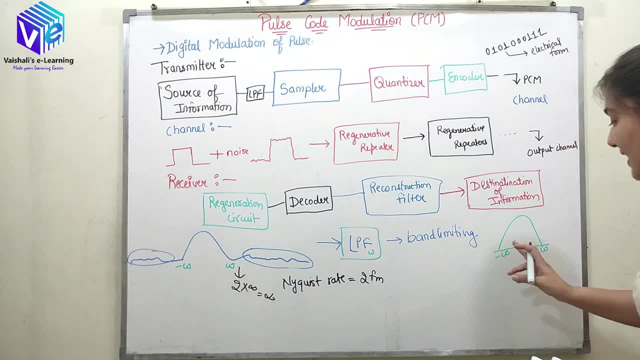 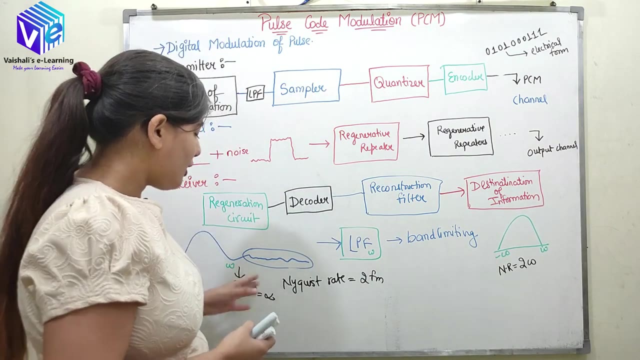 here I require the infinite rate, and here twice of the maximum frequency, which is two W. So the Nyquist rate, or the sampling rate, is limited. now, Here, is it possible? No, So now, because this was impossible. So here first we'll do the band limiting with the. 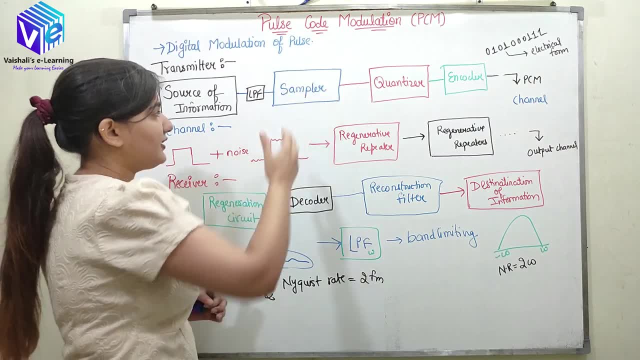 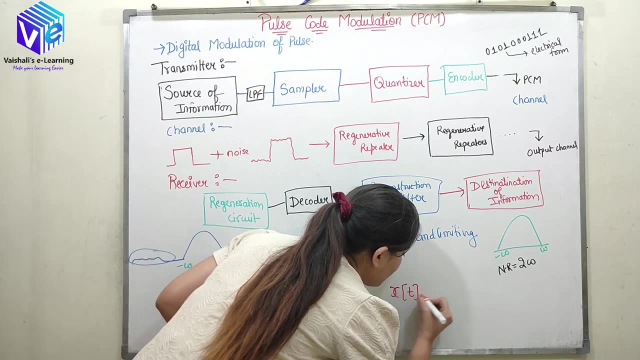 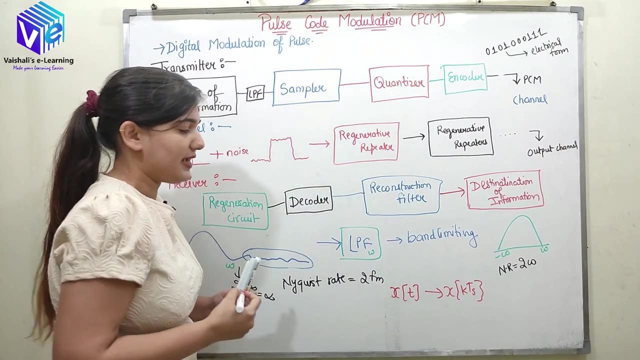 help of low pass filter, and this is called pre processing. After that is fed to the sampler. I hope you remember what is sampling. So if I have signal X, T, it is converted into X, K, T S. So now T S is my sampling instant, So sampling time. So now. 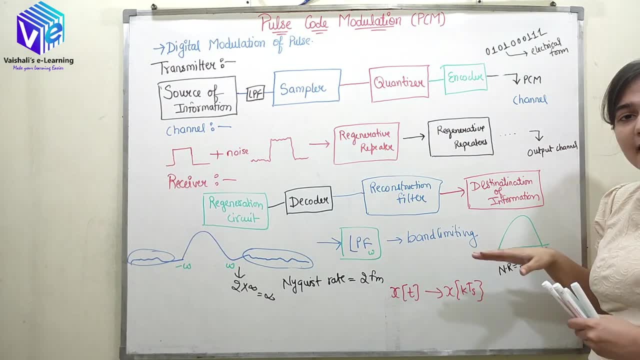 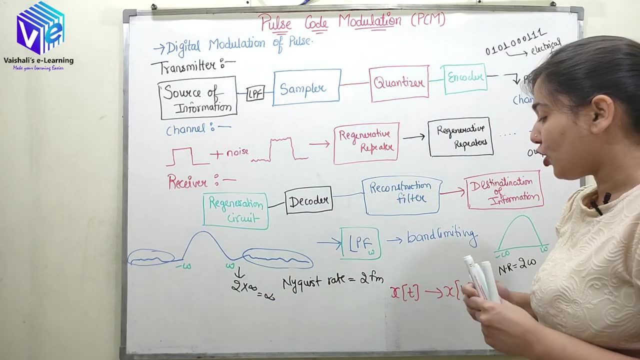 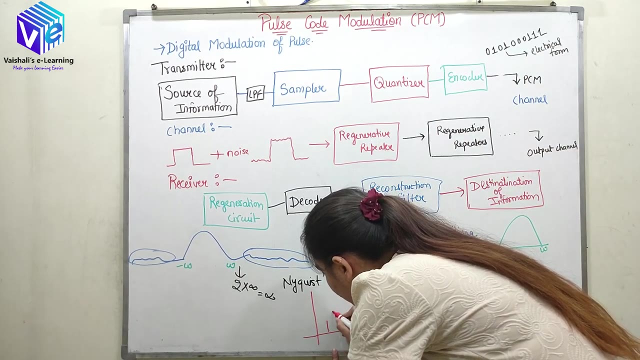 here the sampler is converting the analog time axis into discrete time axis. After that we have the quantizer. So the quantizer, as I already said, it is converting the analog amplitude value. So let's suppose I have a signal like this We'll be talking about. 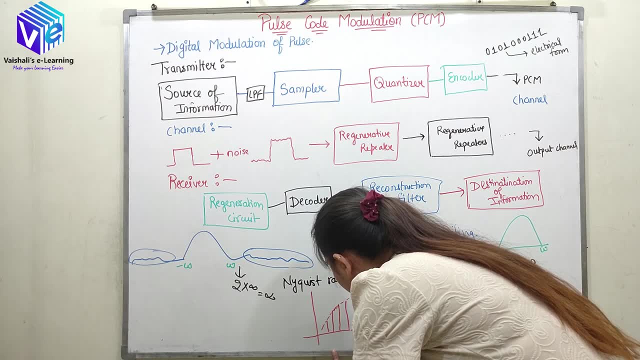 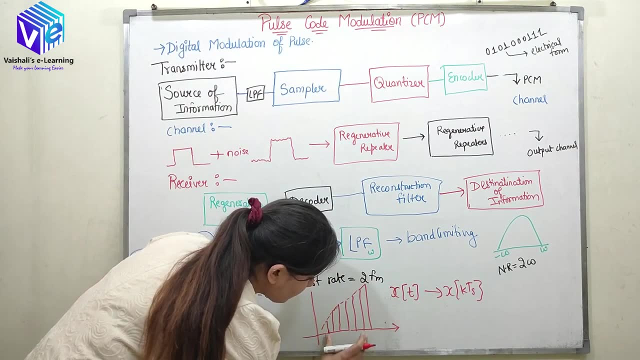 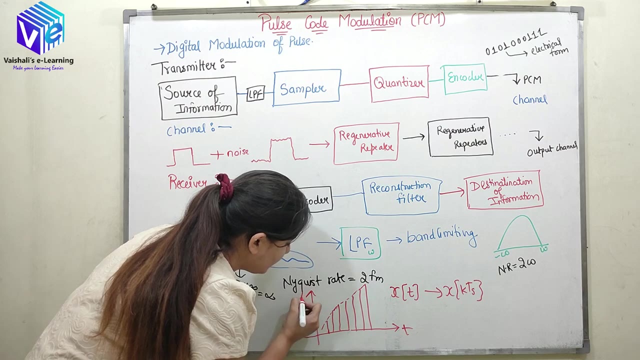 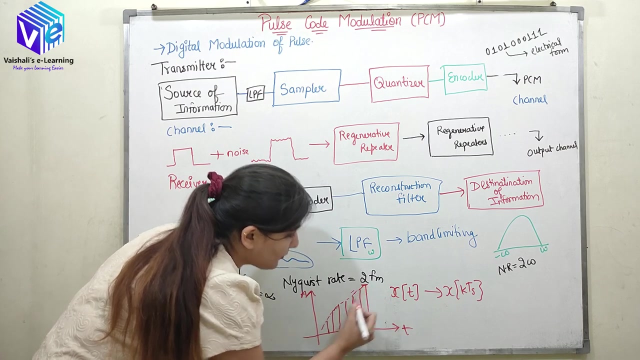 quantizer video as well. but let's suppose this is my signal. here we have the discrete time, so we have already discretized the time with the help of sampling. so now, if i talk about the amplitude, so here the amplitude has every possible values. so if i talk about this amplitude, this amplitude can be like: 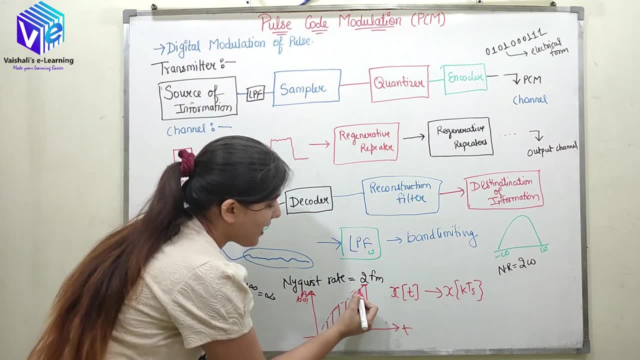 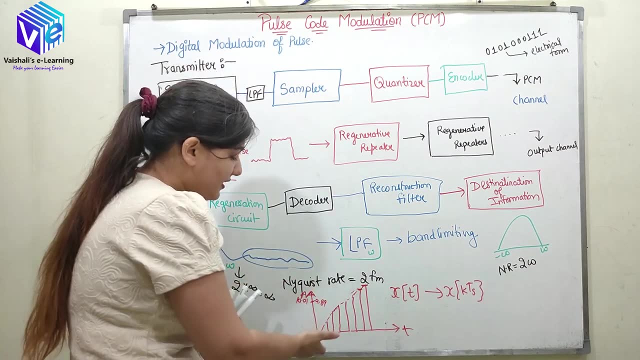 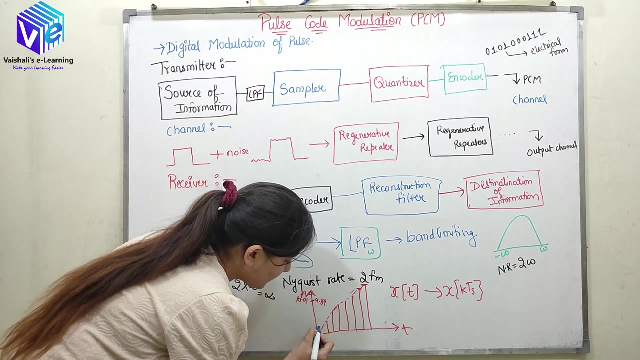 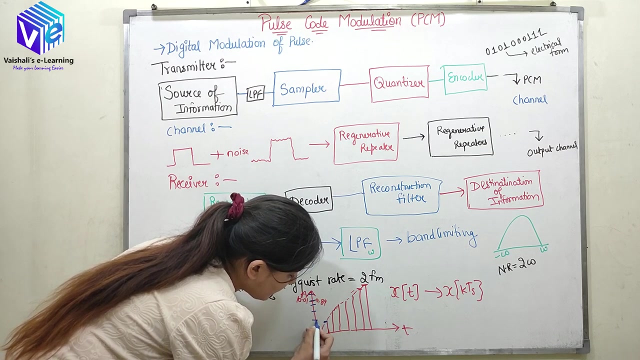 it can be 10.01, or this amplitude can be 9.89. so now we have infinite range of amplitude, or i can say amplitude is changing in analog manner. so now what i can do? i can assign discrete levels. so if my signal is in between this level and this level, so i'll assign either this level. 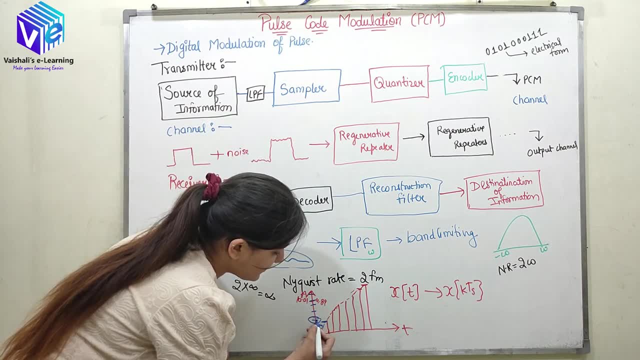 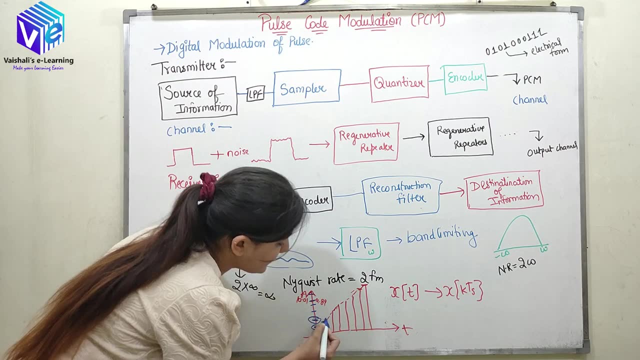 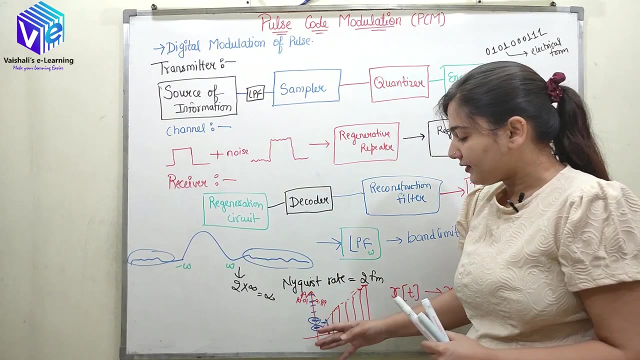 or this level to my signal. so because this is near to upper level, so i'll apply this signal to the upper level. so now this signal is represented by this level only. no intermediate level is allowed. so now i am shifting the signal from infinite possible amplitude levels to finite amplitude levels. 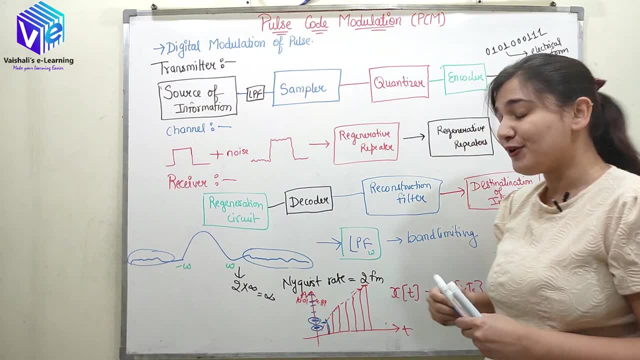 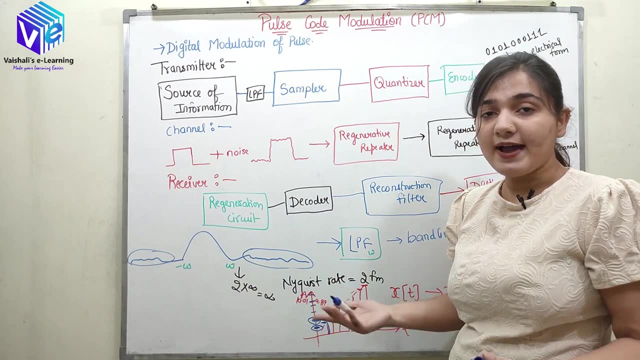 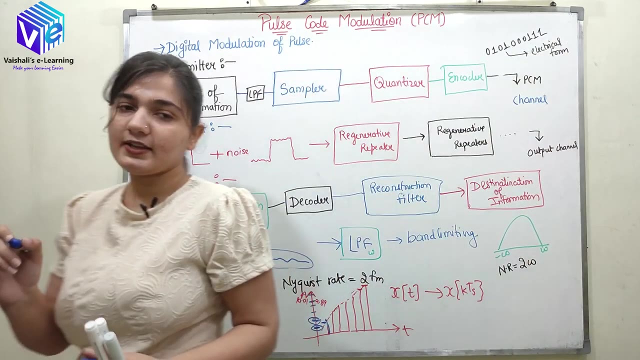 so this is the process of quantizer. now you must be thinking that if i am changing the amplitude amplitude, i am producing the error in the signal myself. yes, i am producing the error in the signal myself. so let's suppose- so here i'll be making it. so let's suppose this was my signal and this is my signal. 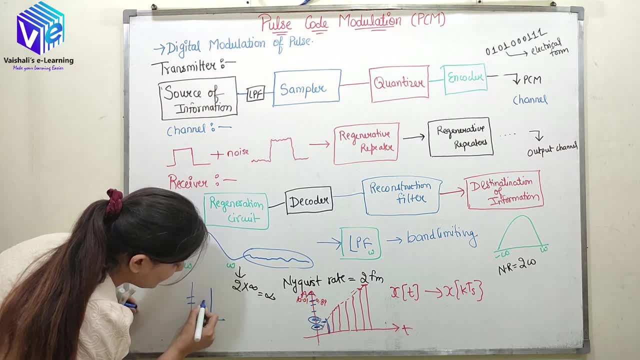 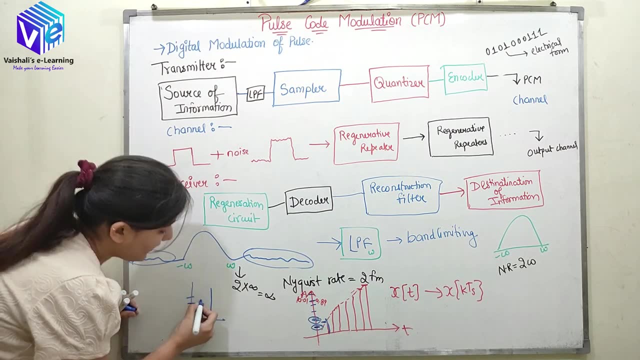 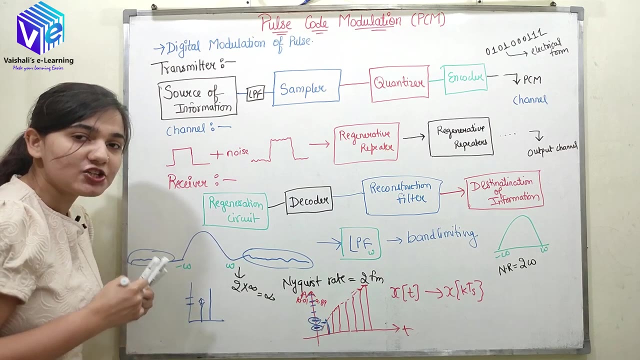 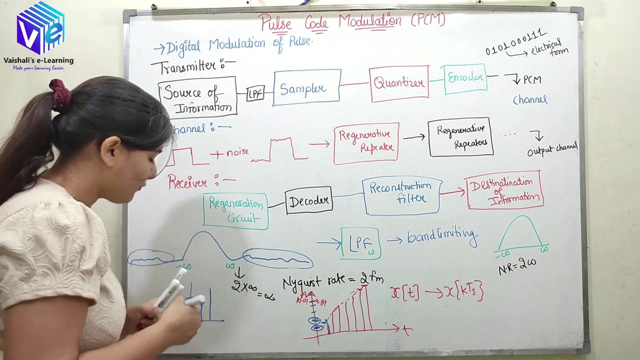 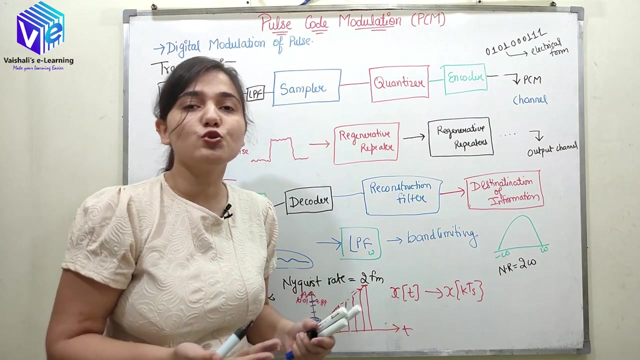 so here, if i am providing this signal to this level, so here i am changing the amplitude level. so here, from here to here, this term is quantization error. so it occurs because we have quantized the signal, now we have changed its amplitude value. so now, how we can eliminate it? we can not eliminate it, we can just reduce it. how? 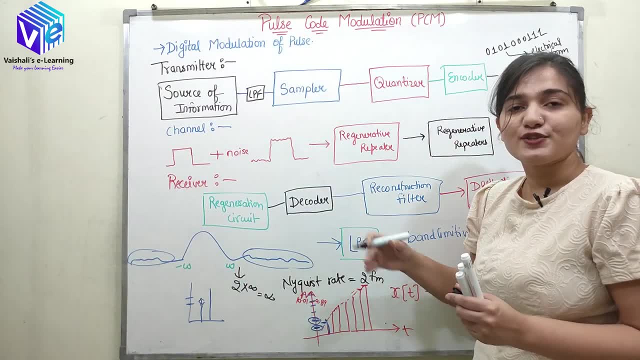 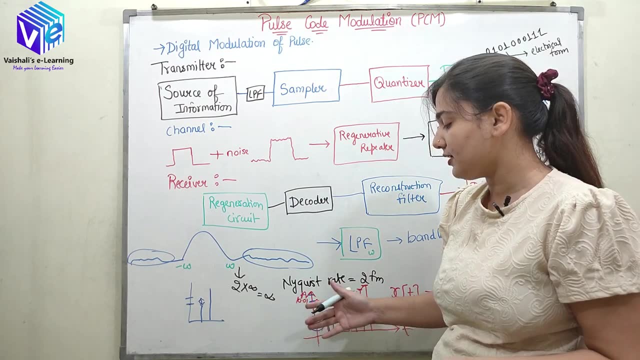 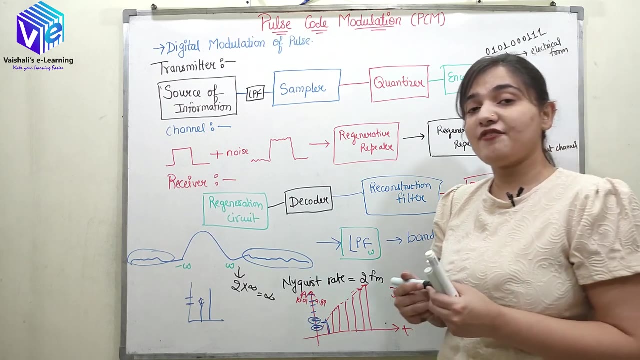 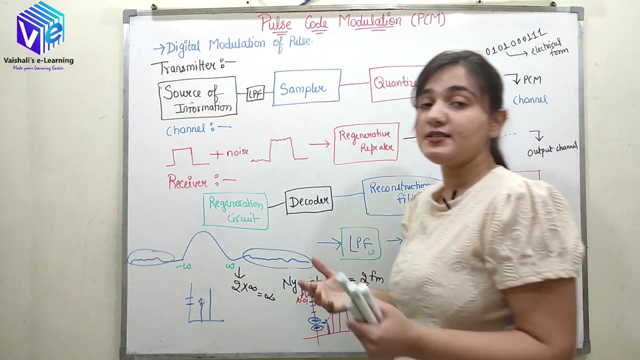 if i am choosing more number of levels, so the quantization error would automatically reduce. so here instead of like, let's suppose, instead of four levels, if i choose eight levels, so the quantization error would reduce. but what happens? if i choose more number of levels? the next block would produce a problem. so the problem is that if i have more number of 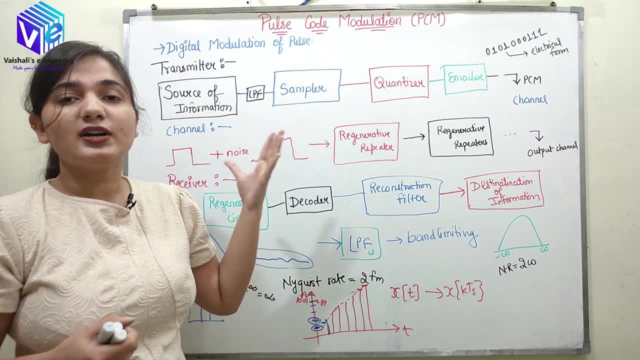 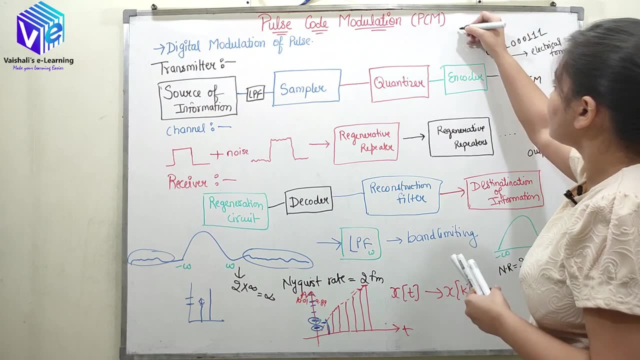 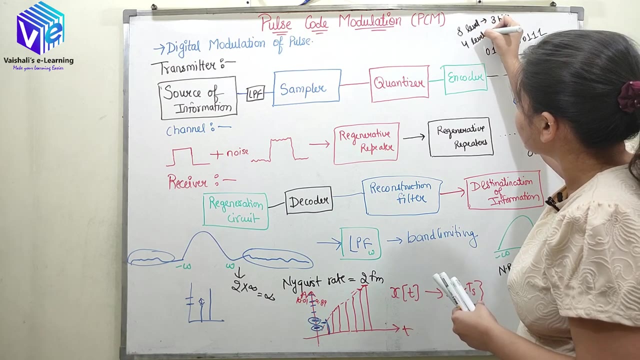 levels, i require more bits to encode a given signal. so if i have, let's suppose, eight levels, so eight levels are encoded by three bits and four levels are encoded by two bits. so if i have four levels, only two bits are required, which are zero, zero, zero. 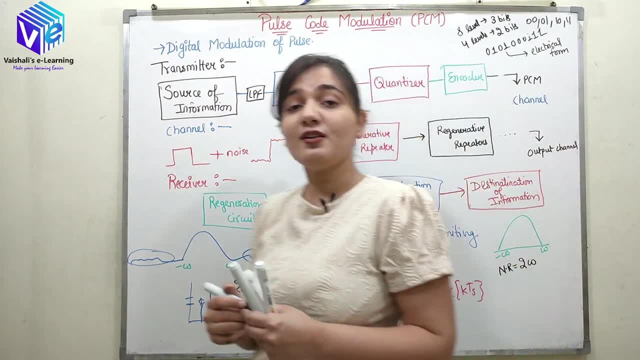 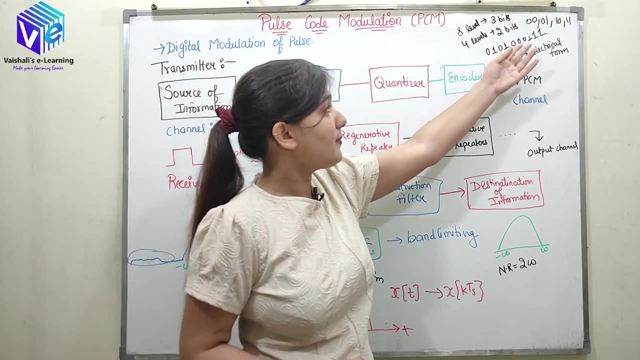 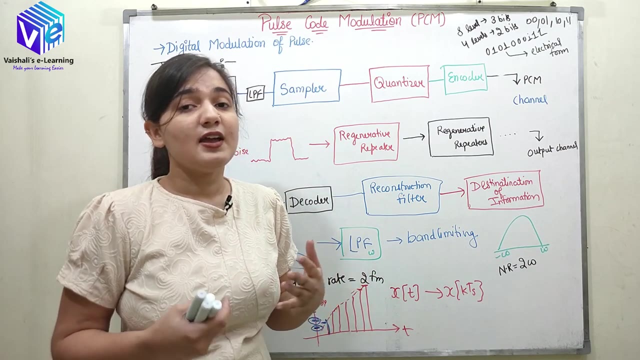 one, one zero and one one. i hope you know this. so if i am myself making more levels, the encoder will be having more number of bits. when we have more number of bits, the transmission frequency would be increased. so now the frequencies when the frequency will decrease. if 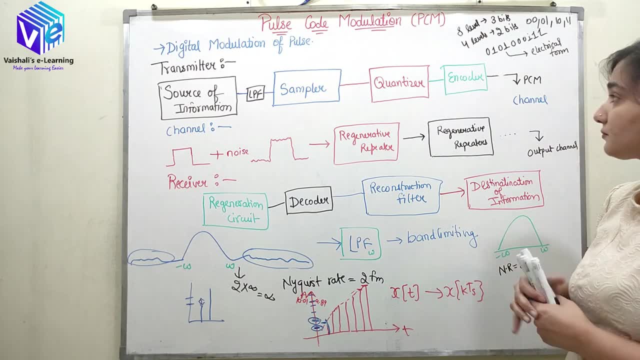 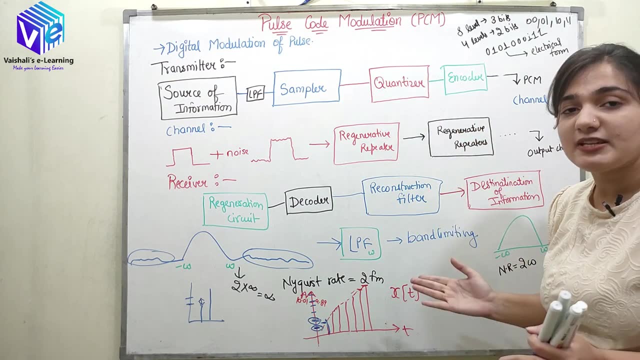 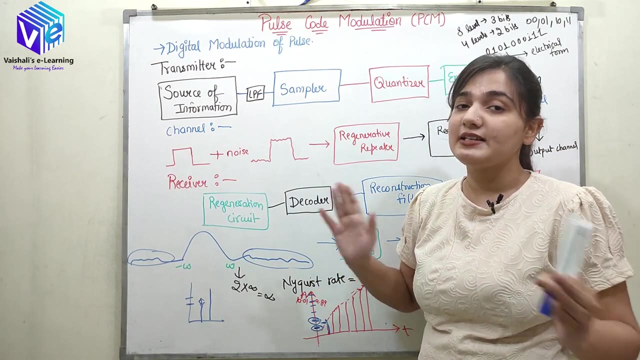 frequency would be increased. the process become costly. So now, to avoid that, we require the quantization levels to be minimum, as minimum as possible. We cannot minimize them after a threshold, So we cannot increase them beyond a threshold as well, So that the frequency 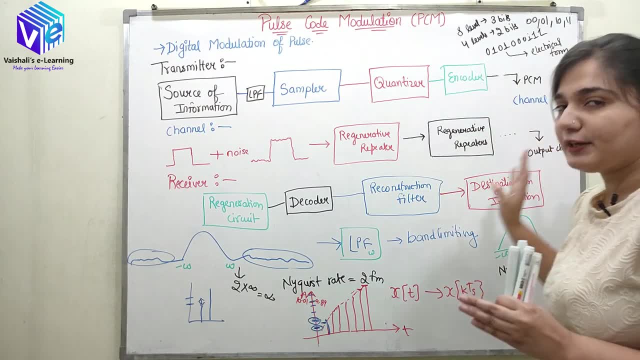 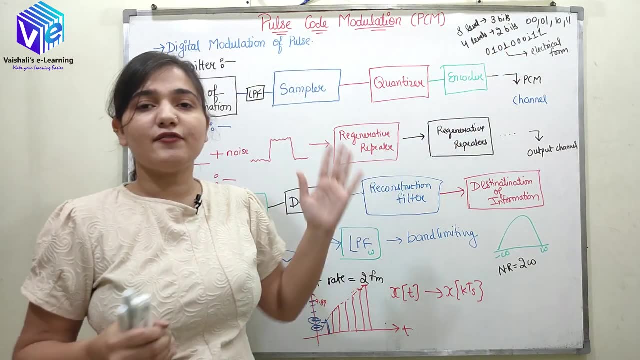 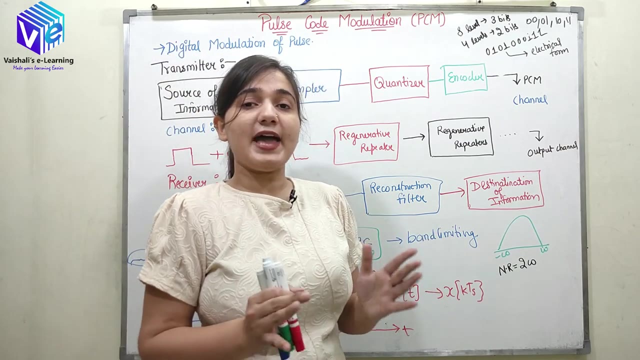 requirement would be less. So now, after that, it is fed to the channel. After that we have, I hope you remember- in the encoder we are converting the signals in the form of zeros and ones. plus, in the encoding we are adding the parity bits. So what are the parity bits? The 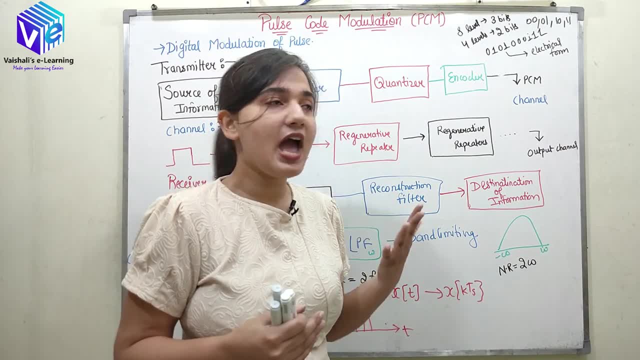 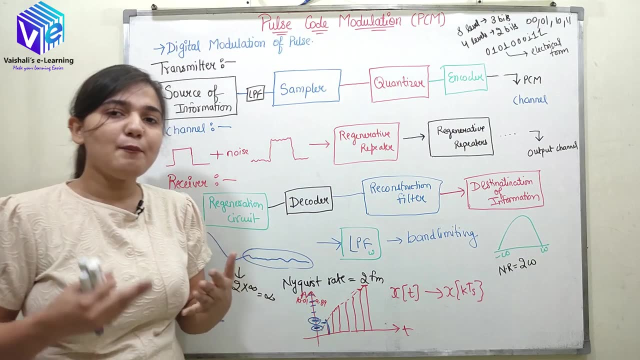 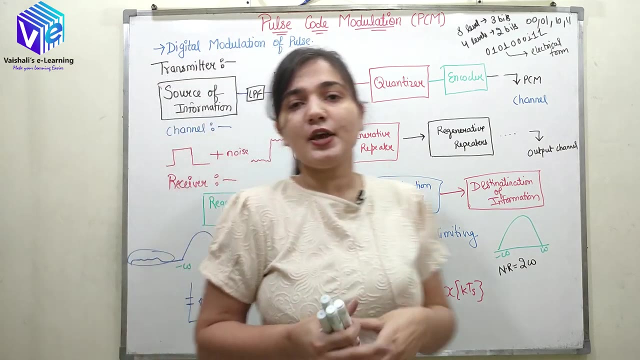 parity bits are required for the error detection and correction. So after that these are converted into the electrical form with the help of line coding techniques. I hope you remember that in the channel, as I said, there would be noise Which is getting superimposed. So here we have regenerative repeaters. What happens in the 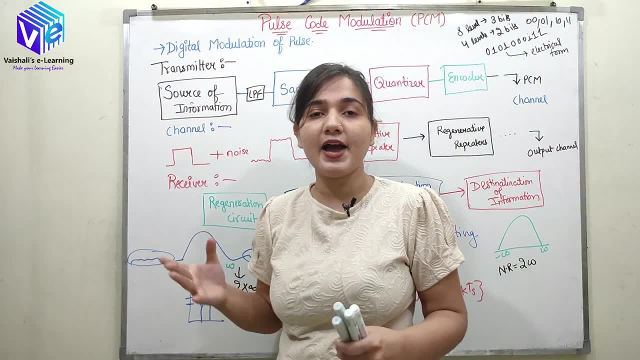 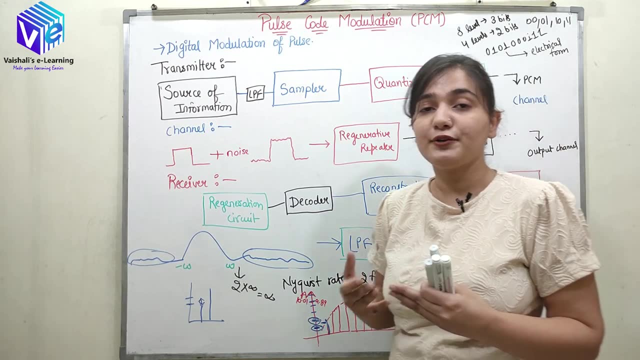 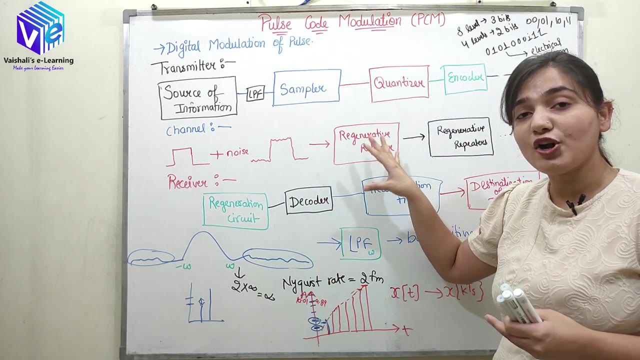 regenerative repeaters. So here, due to noise, we will be having the amplitude errors as well as phase delays. So I have already talked about the aperture errors, So you can remember that. and, like the same way, we have the distortions in the amplitude as well as phase errors as well. So 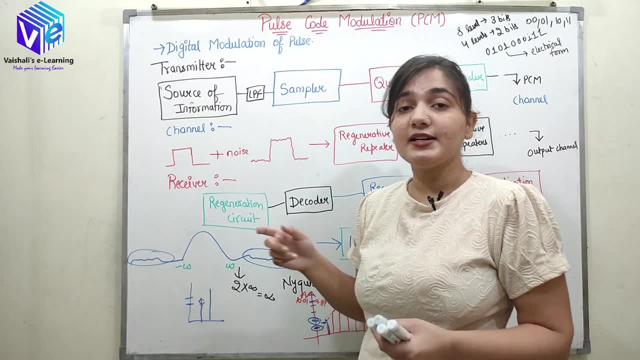 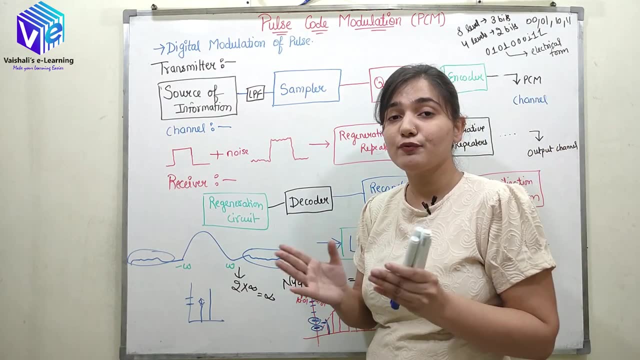 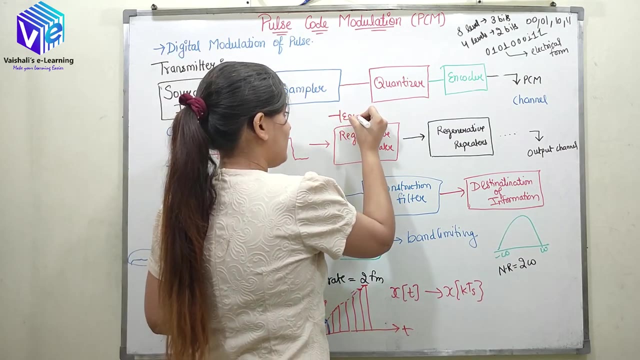 to remove that, we have regenerative repeaters, And in the regenerative repeaters the first block is equalizer. So equalizer is removing the effect of the amplitude and phase distortion. So here we have equalizer Now. after that we have 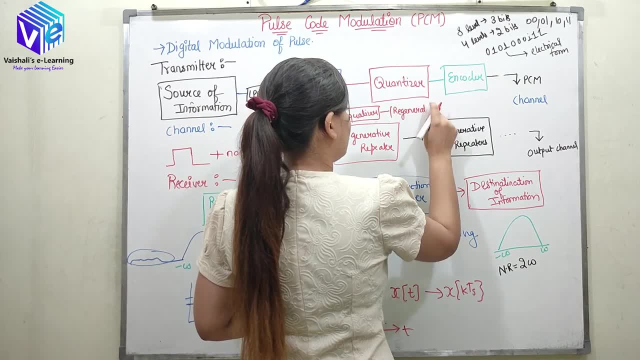 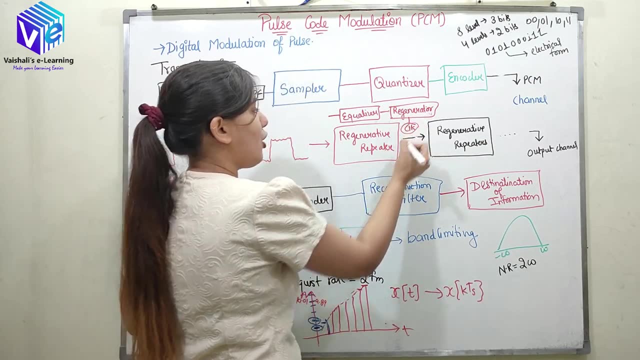 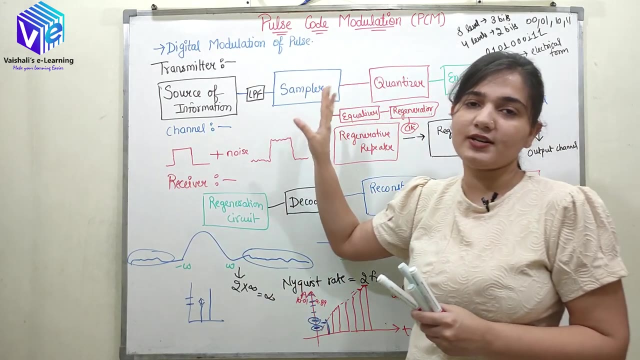 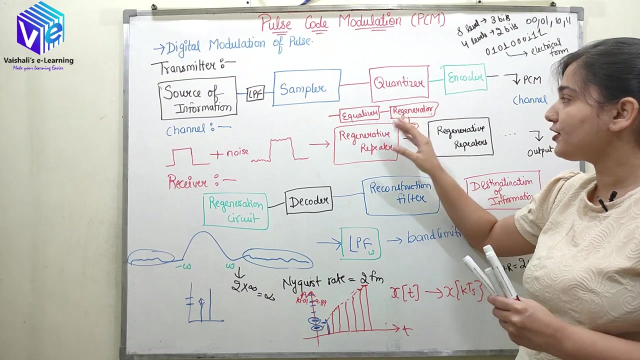 regenerator. So now the regenerator is having the clock, which is the same clock, the transmitter. so what happens? the equalizer will remove the phase distortion, as well as amplitude distortions, as much as possible, but what happens? all of them are not removed. so now 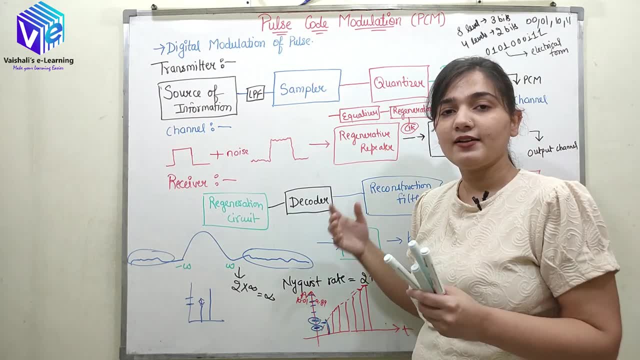 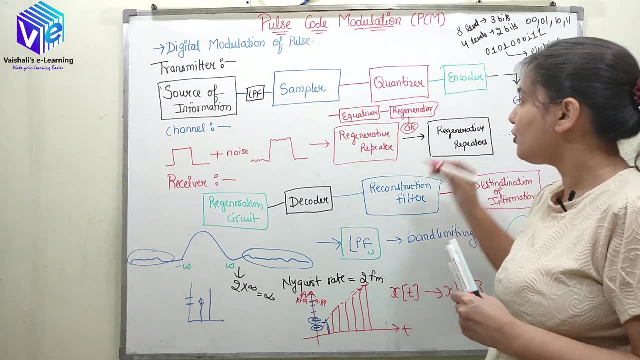 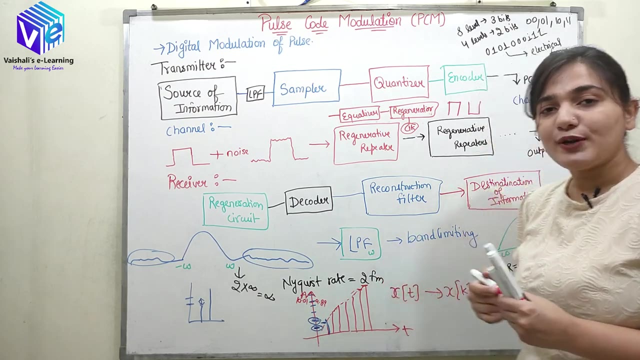 what happens in regenerator. again, we will check with the help of the same clock whether the signal transmitted is having positive value or negative value. if it is having positive value, we reconstruct one. if it is having negative value, we reconstruct zero. so now again i'll be having after the 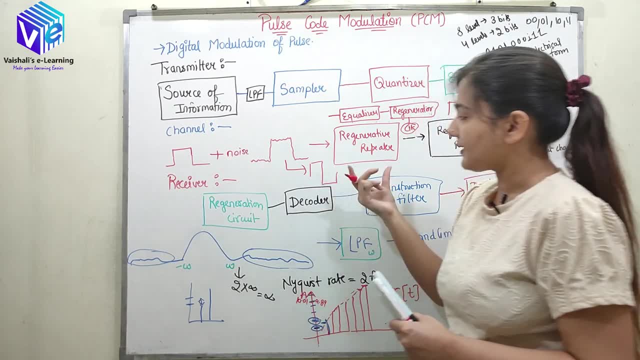 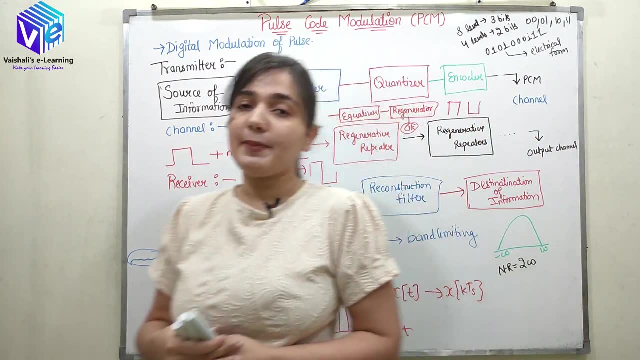 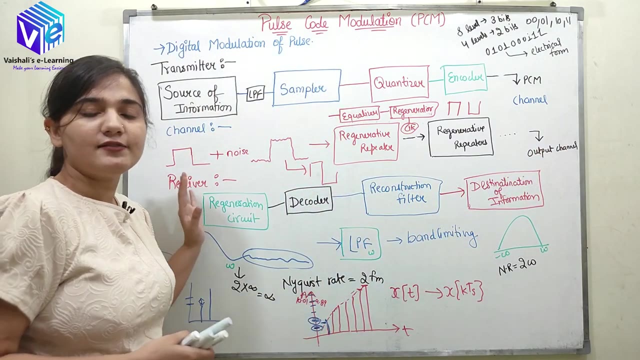 regenerating repeater, i'll be having the exact output. so now again i'll be having various regenerative repeaters, depending upon the need. after that it is fed to the output of the channel, and at the output of the channel we have the input of the receiver. so in the receiver, the 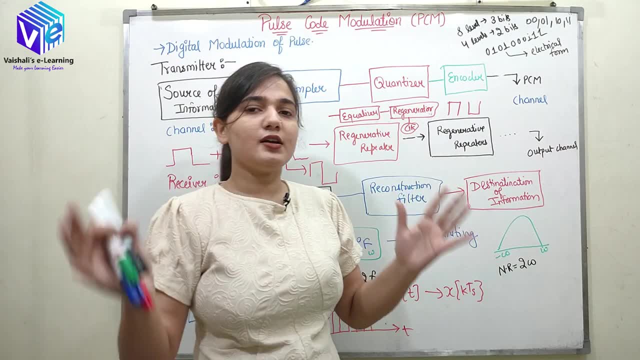 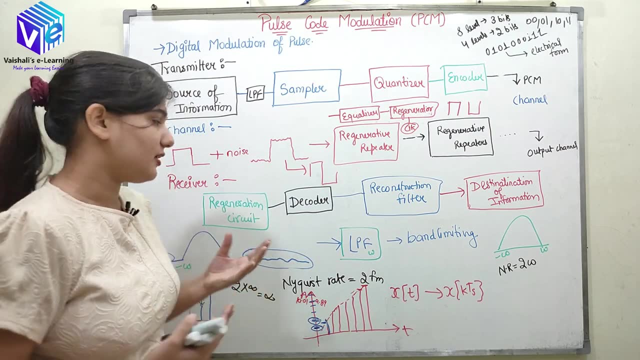 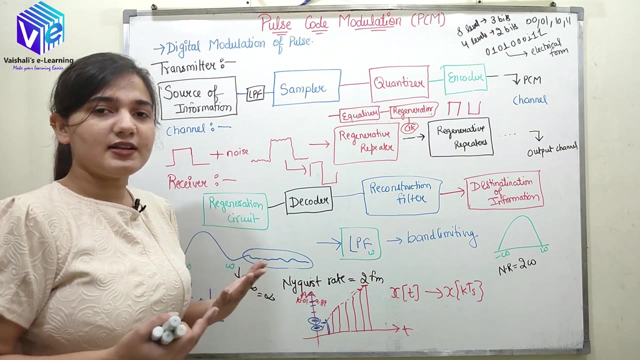 first block is regeneration circuit. so the signal which we have received, because we have not done any kind of modulation, so there would be more tampering in the signal. so now in the regeneration circuit again i'll be doing the same thing. we'll try to regenerate the signal with the help of equalizer. 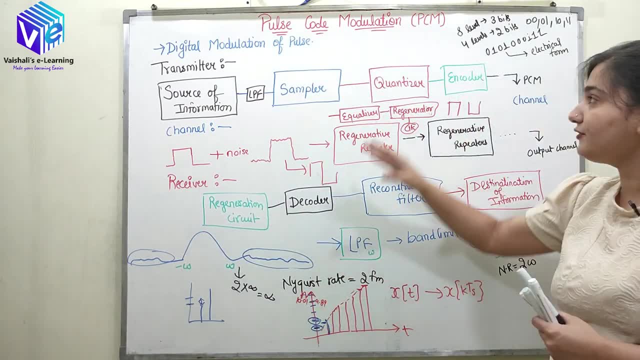 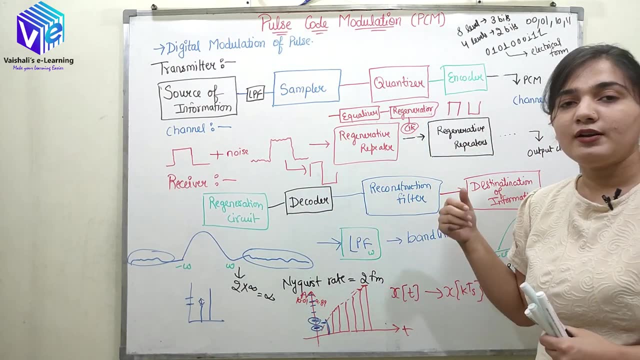 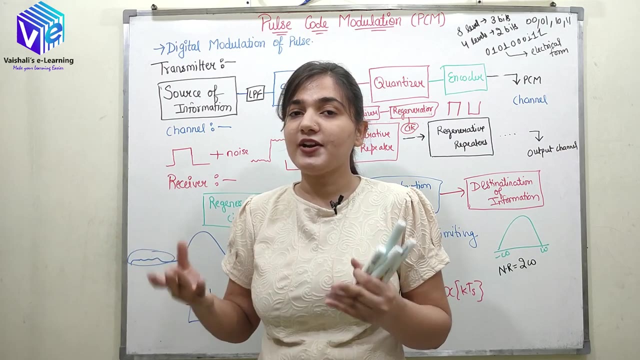 and the regenerator. so after that we have the reverse of these blocks. as i said, encoder is the reverse block of decoder. so in the decoder what happens? the parity bits are removed and we check that if errors has occurred or not. if it has occurred, it will correct the error or it will ask.